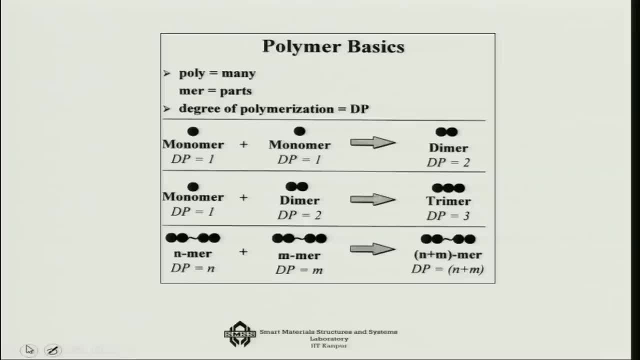 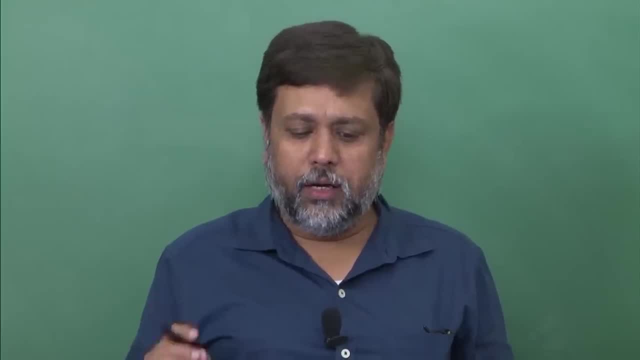 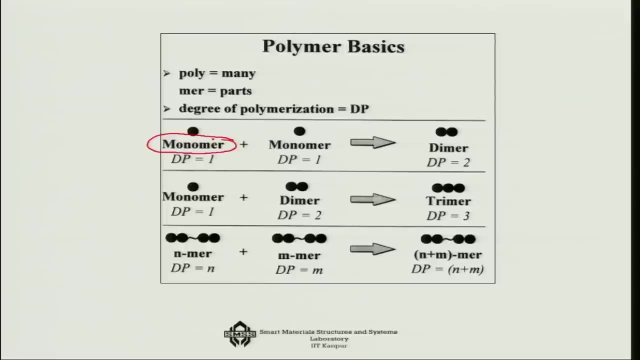 know that Greek part in it, where the poly means many and mer means part. So that means whatever polymers. you see, it is essentially made of many, many individual parts. Each one individual part is actually called a monomer, a single part. Now, once I consider two monomers: 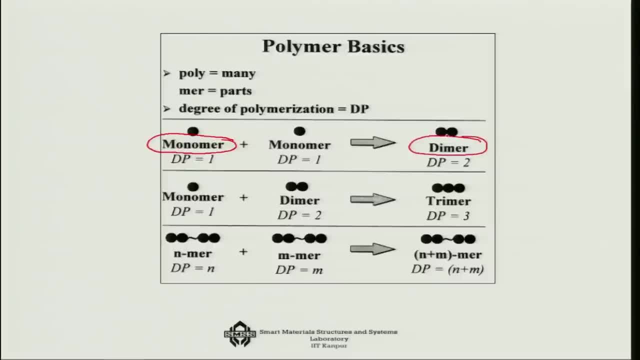 together, if they join their hands, then they become a dimer, So a monomer. also, by definition it has a degree of polymerization, or dp, which is 1.. Now, if there are two monomers, then the degree of polymerization becomes 2.. So for dimer it will be degree of polymerization. 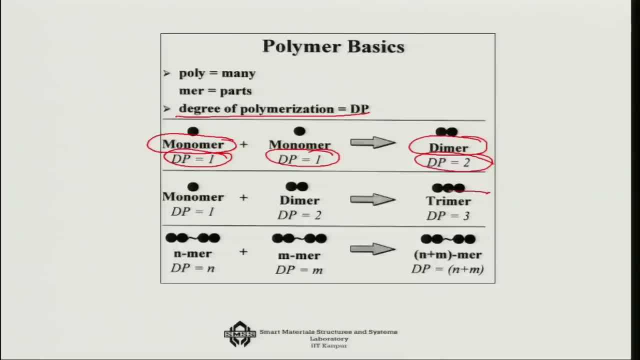 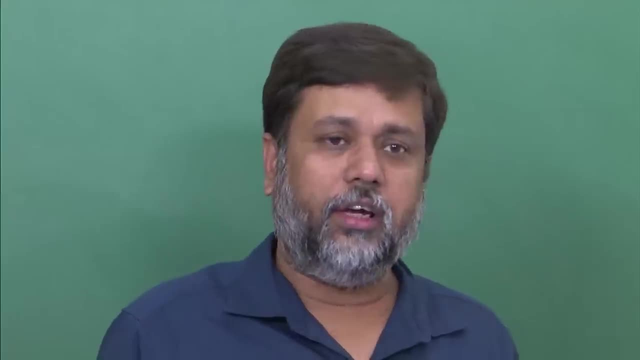 which is 2.. And monomer with a dimer, you will get a trimer and a degree of polymerization will become 3.. Of course, this one unit, one unit adding together, or such kind of very, very small number of units happen, for you know materials like silicon, in which there is a term called oligomer. 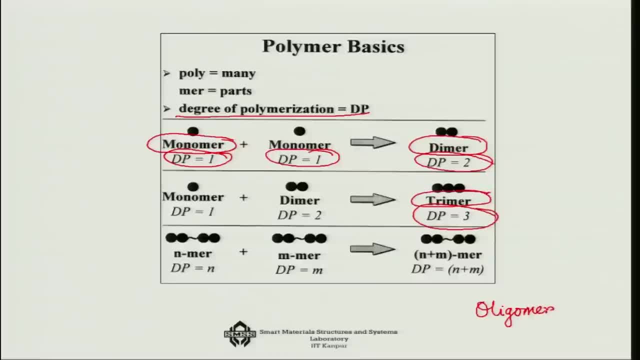 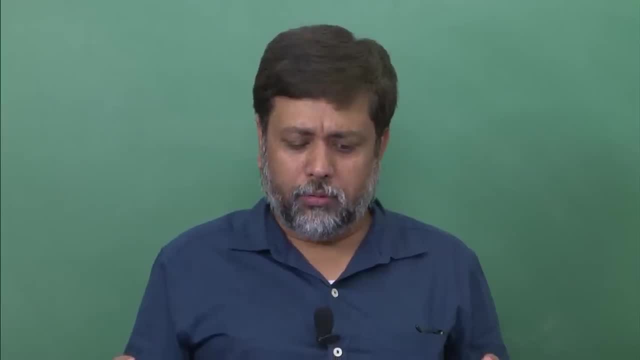 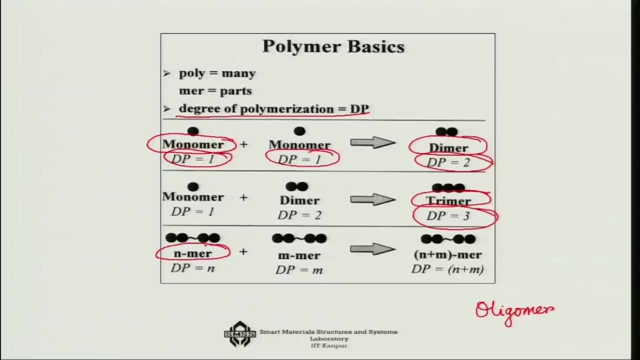 So that means you know there are something like 5,, 6 or 10 of the monomers join their hands together, So you get a n-mer with a m-mer, two such polymers when they add together, concatenate. 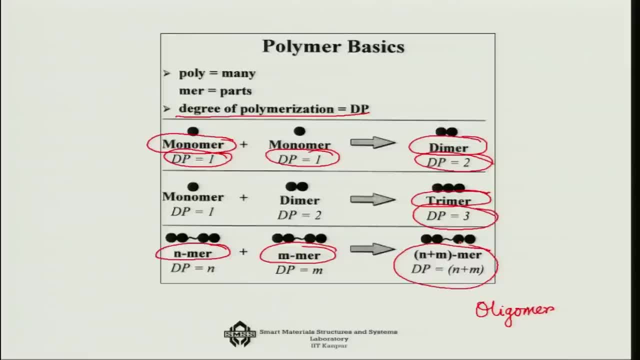 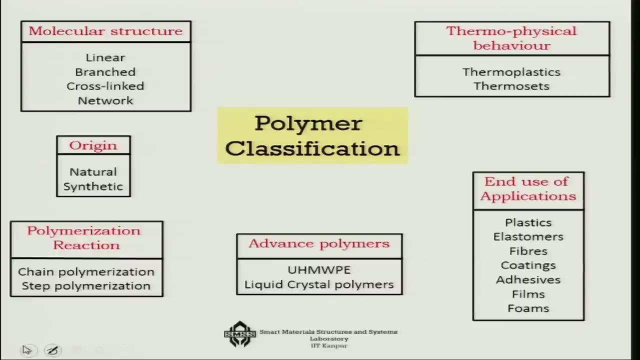 then you get something like a n plus m-mer with a degree of polymerization of n plus m. So that is the kind of a very big scale polymer that we are talking about. Now, how do we classify the polymers? There are various ways in which we can classify. 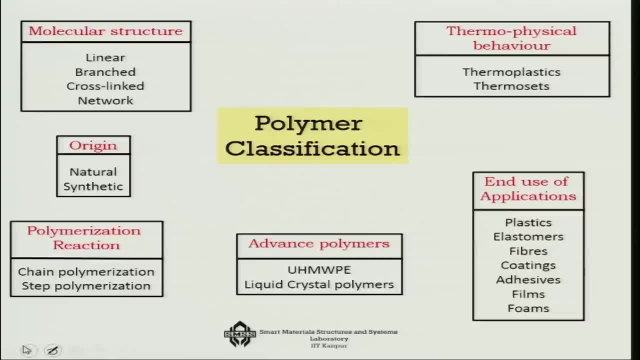 the polymers. We will discuss them one by one today. For example, we have a polymers type and a molecular structure type. For example, you can classify the polymers on the basis of their molecular structure. If you try to do that, I will show you that it starts with. 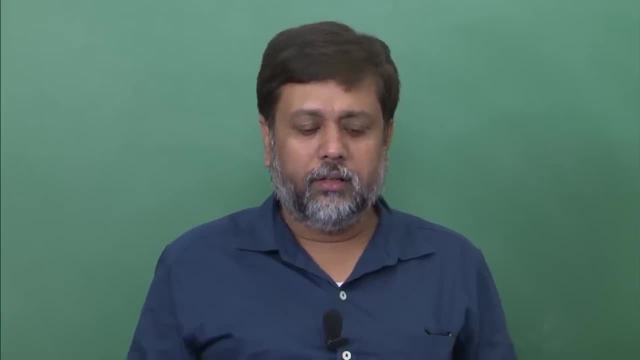 the simplest molecular structure, where it is completely linear. Then it can be branched. that means some branching coming out of the linear. Then it can be cross linked. that means the branches are chemically linked and then it can be networked. So that is the molecular 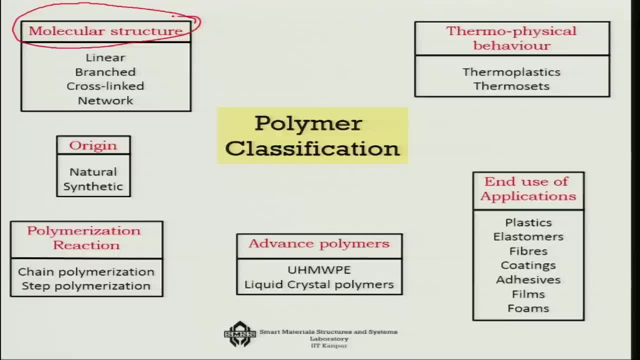 structure wise. If you look at it from the origin point of view, you can very simply divide polymers into two types. one is the which is having natural origin, So natural polymers and synthetic polymers. So that is this group. and then from the polymerization, 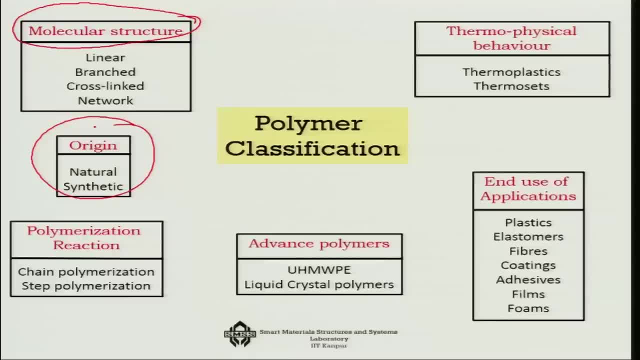 reaction point of view. that means how the polymer is developed. if you look at it, then two most important types are chain polymerization and step polymerization. So that is from the polymerization reaction point of view, Then from the thermo physical behavior point. 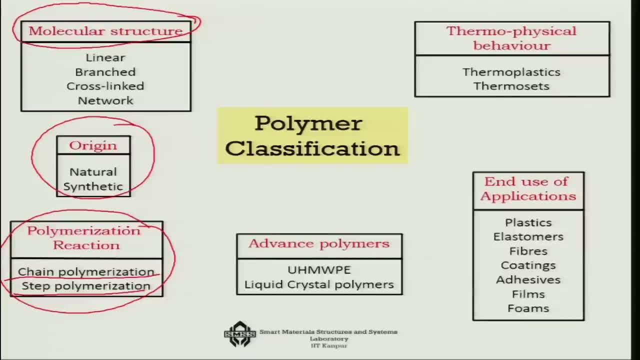 of view, we generally classify the polymers into two groups. one is the tachy, so called, you know, polymers, which can, actually you can give it many kind of forms, So that is thermo plastics. and the other group which, with respect to temperature, you can give it a set form. 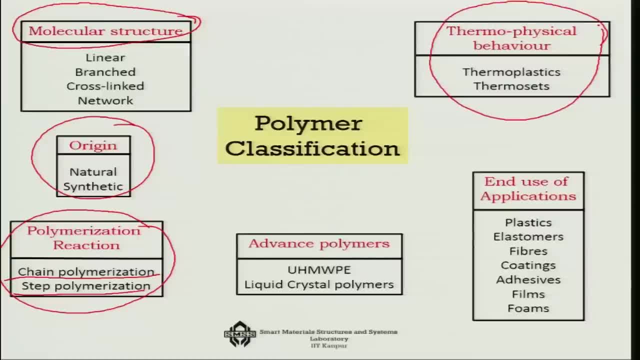 that is, the thermo sets. So that is another way of classifying the polymers. Then, in terms of the applications, there are end use of applications of polymers. that is also another way looking at polymers and there are some polymers which are actually advanced polymers. 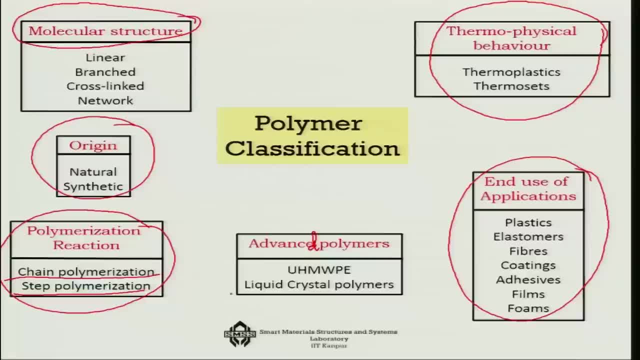 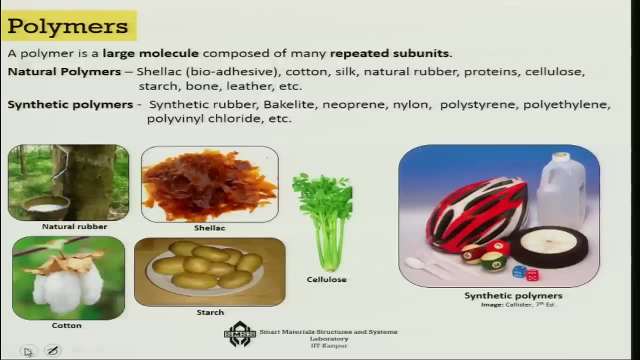 So this advanced polymers, so that is, like you know, UHMWPE, or liquid crystal polymers. that is like some of the advanced versions of the polymers. So let us try to look at them one by one Now from the- you know- the origin point of view. if you look at the polymers, then you 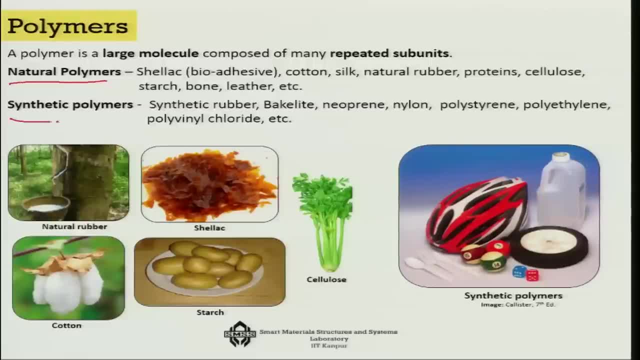 can. I told you that you can divide into two groups: natural polymers and synthetic polymers. Natural polymers are like the shellac or bio adhesives. ok Say, for example, you can consider some of the latex of the tree that comes out, or the 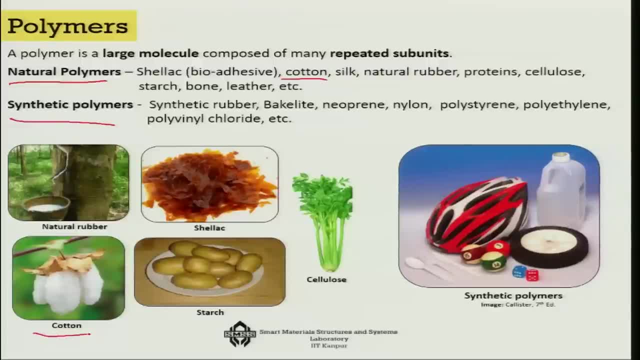 cotton, the cotton or the silk, ok. natural rubber, ok. shellac, of course I told you. and then the starch, which you get from potato- ok. Or the cellulose that you get from some of the plants. these are all some of the examples. 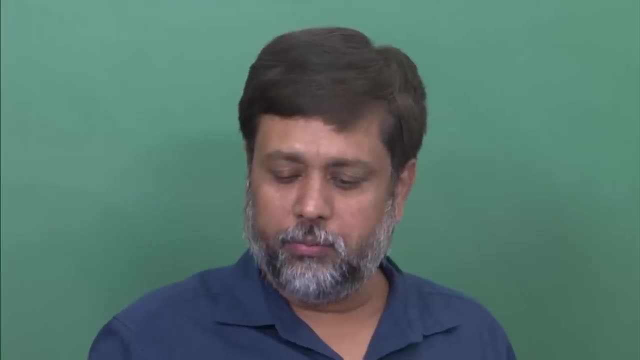 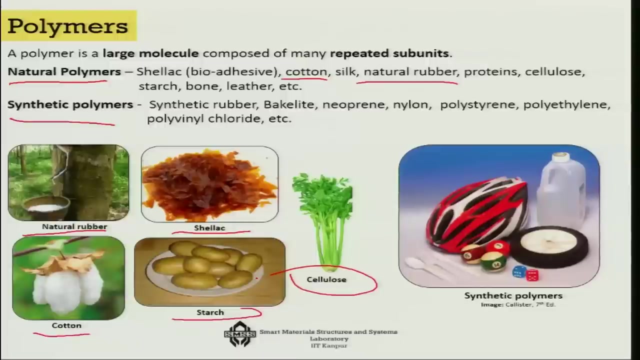 of our bone itself. some of the examples of natural polymer And some of the examples of synthetic polymer. our world today is actually surrounded by all sorts of synthetic polymers, like synthetic rubber, dacrylate, neoprene, which is also a form of rubber, nylon, for example. polystyrene, polyethylene, PVC's, polystyrene, polystyrene. 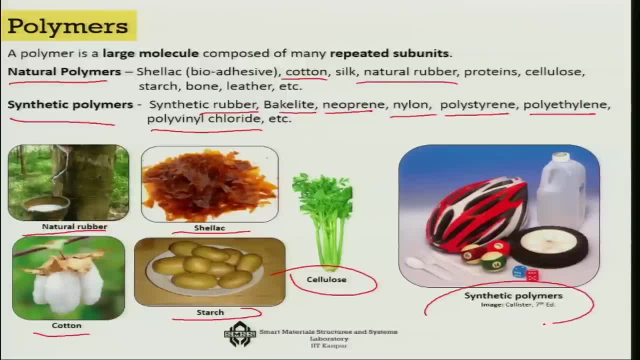 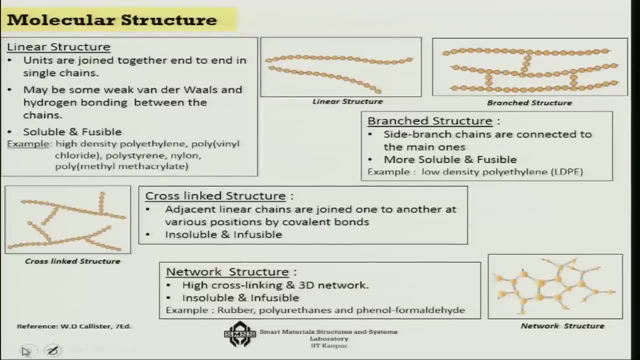 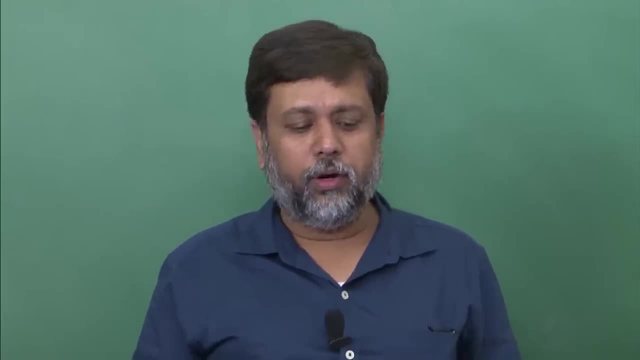 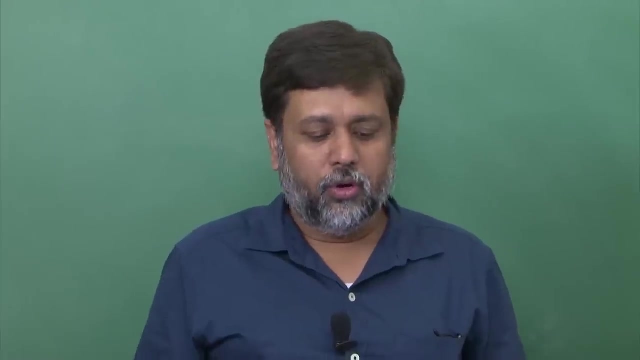 polystyrene. So there are so many of them, the synthetic polymers. ok, so that is as far as the origin of the polymer goes. Now, if you try to divide it in a different way, more like a- you know, fundamental point of view, then you can actually characterize polymers in terms of their molecular structure. 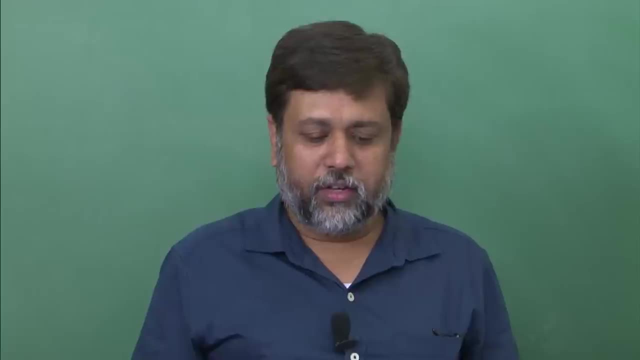 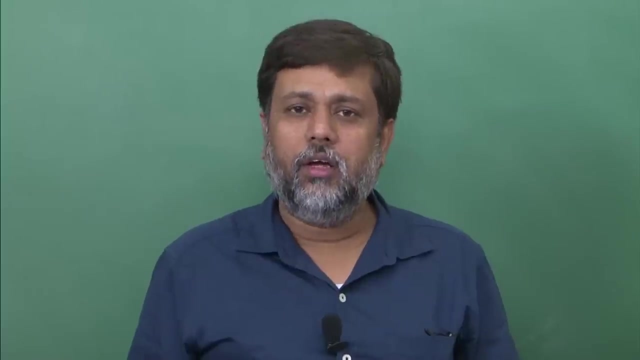 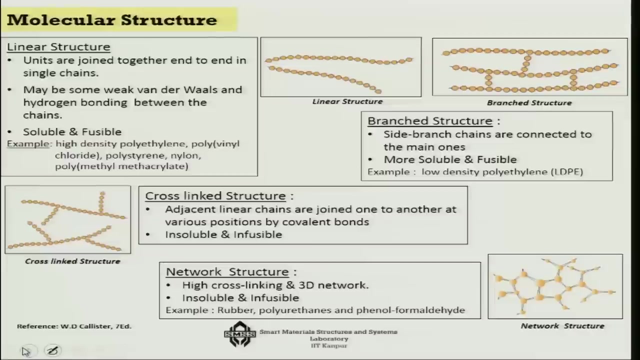 So that is something that is little more advanced than you know in terms of, instead of dividing them In terms of the origin of the polymers. so here, what you will see is that the polymers are essentially of three types, that is, the linear polymers, then the branched polymers. 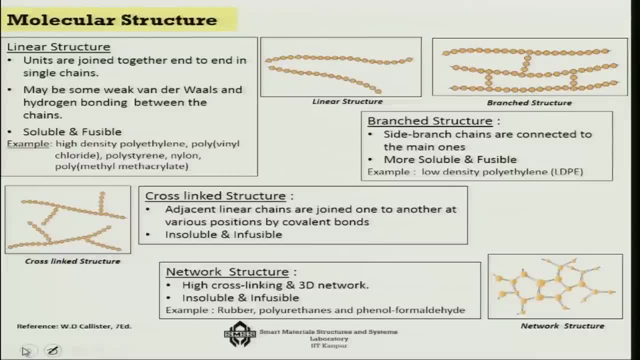 and then those which are chemically linked. in fact, out of them, there are two types. we call it. One is actually then when there is a cross linked structure, and another is when there is a network structure. So, to begin with, we will first see the linear structure polymers. 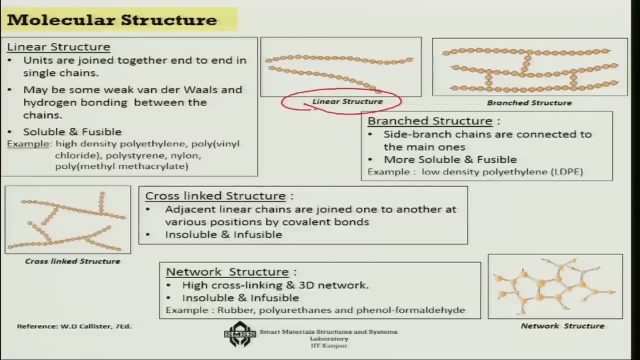 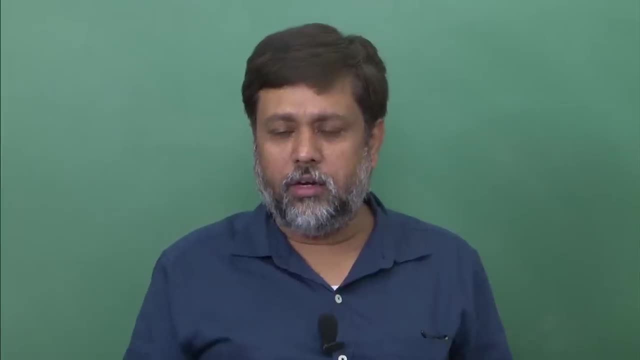 So some polymer units are just like monomers, joining their hands together and building up their longest chains. ok, Something like polyethylene. polyethylenes are so single units of ethylenes. you just add them all together, you get a long chain: polyethylene. 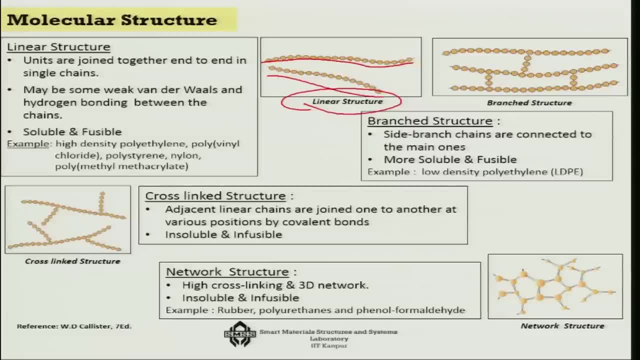 This are, you know, the each one of them. of course, along their axis, because of covalent bonding, they are very, very strong. ok, But if you think of the transverse direction between the two, then there is not much of a you know a bonding force there. 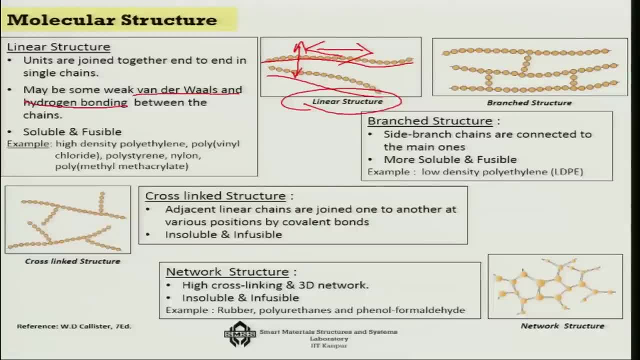 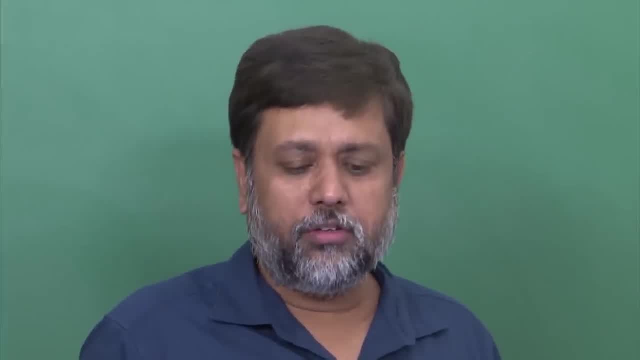 This will be either very weak Van der Waals bonding or hydrogen bonding kind of things. So as a result, they have first of all, directionality. in one direction they will be exceptionally strong and high modulus of elasticity. on the other hand, in another direction, they would 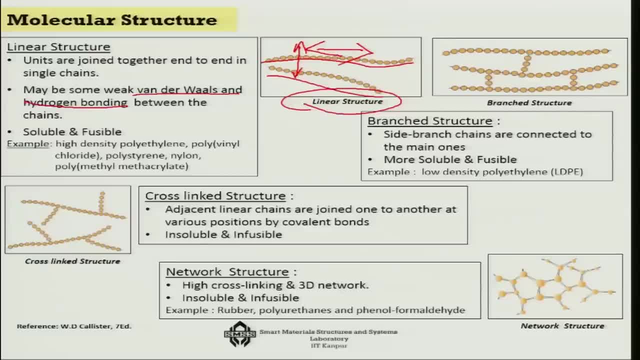 not be So they will be weaker And they are soluble. they are fusible because of this kind of structures and they are green also, you can use them many a times. that is why polyethylene- you know the films- you can actually reuse them or recycle them very easily. 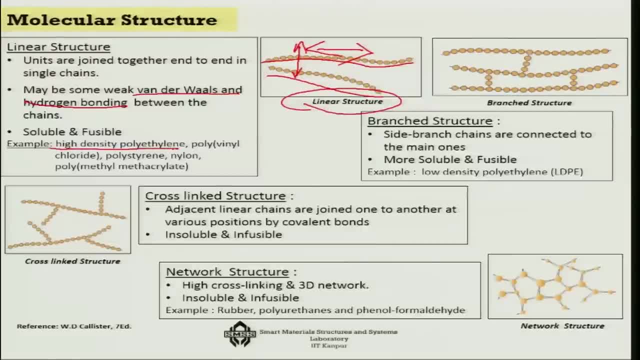 So the examples are like high density polyethylene, low density polyethylene, etcetera, And then PVCs, polystyrene, nylon, you know, PMMA. all of them are good examples of the linear structure. The other point is that linear structure also. generally they have actually good what you 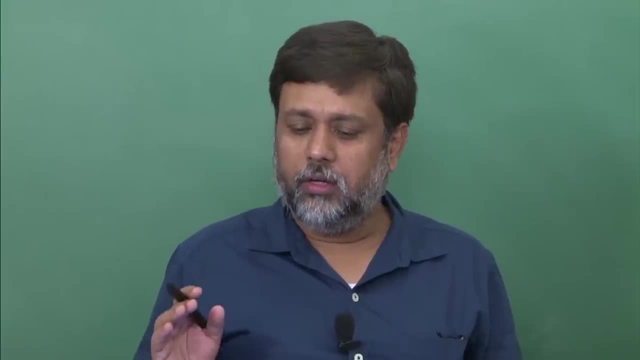 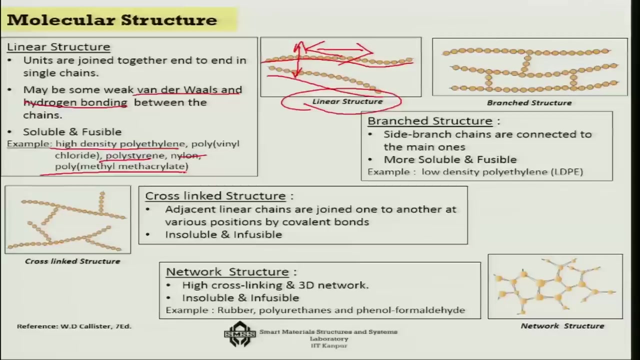 call the crystal structure. ok. So because their repetivity is generally very good and, as a result, many of the linear structures- not all, but many of them- are actually highly crystalline. So the degree of crystallinity if it increases, that also improves the mechanical property. 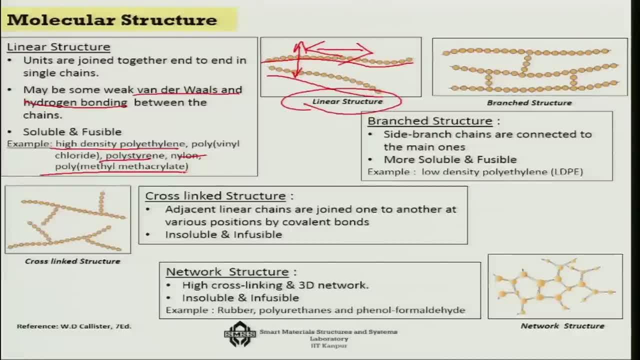 of the system. Now, some of them, the linear structures, are not just linear but they are branched type of structures. So that means there are side branched or chains that are connected to the main ones chemically, ok, But with the another such link there may be only, once again, hydrogen bond, or you know. 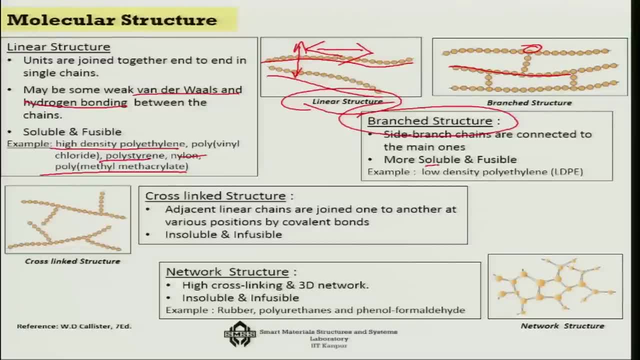 van der Waals bonds, etcetera, So they are more soluble and feasible. And, ah, Some of them are like low density. polyethylene is one of them. So that is ah, linear, but there are some branches with it. Now, if the branches, you know, kind of gets cross linked, so that is what is the cross. 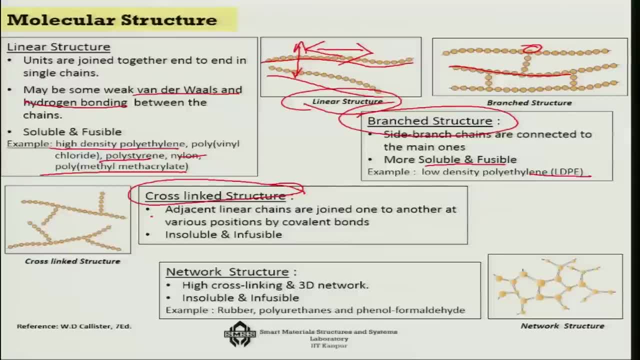 linked structure, then what you are getting is that the adjacent linear chains are joined one to another at various positions by actually covalent bonds, and they become insoluble and infusible. So that is what is the cross linked structure, If this degree of cross linking increases so much that they form a network structure. 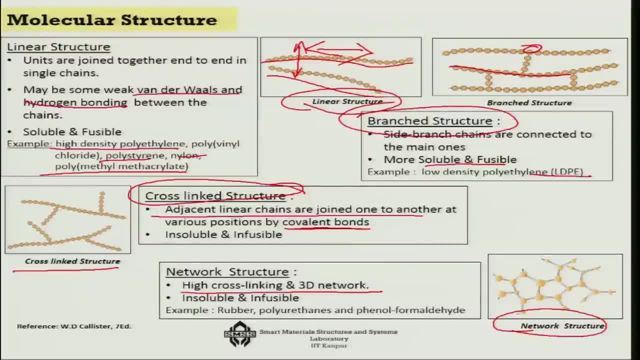 with high cross linking and 3D network, then that is the extreme form of cross linking and this will become insoluble and infusible, like rubber, polyurethane, phenol, formaldehyde or what we normally call epoxy- ok, epoxy resins. So 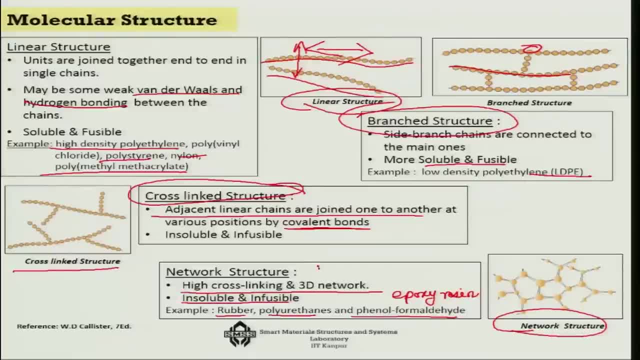 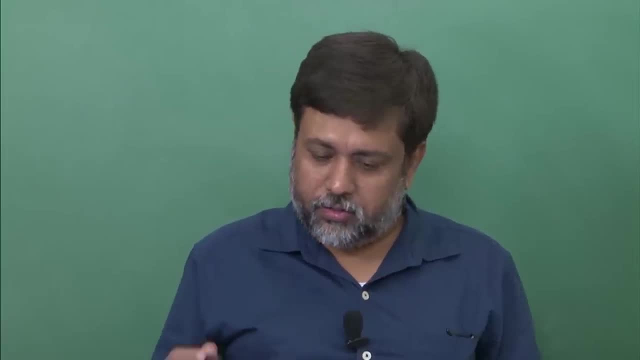 So, So, So that is the- you know- ultimate example of network structure. So this also is important in the sense that cross linked and network structures are actually mechanically more rigid than the linear and the branch structures And there is a correlation between this kind of the you know from the ah, in terms of the 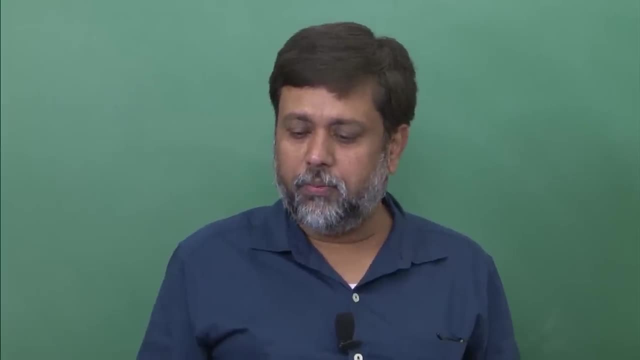 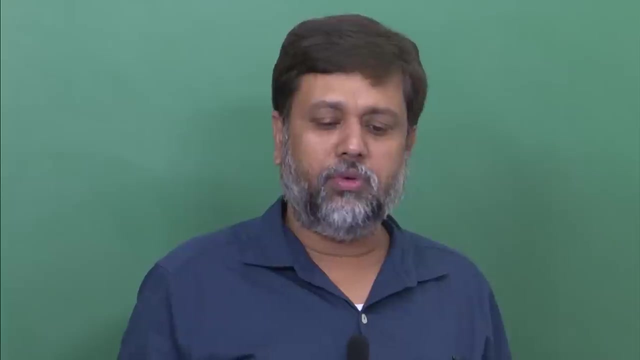 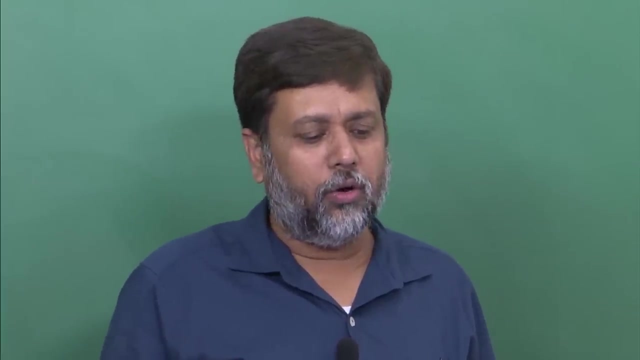 growth of the polymer from the molecular structure point of view and the thermo physical point of view, If you categorize it. there is a correlationship between them and that is, if you see the polymer is, ah, you know, if you find it to be linear or branched, then there is a high degree of 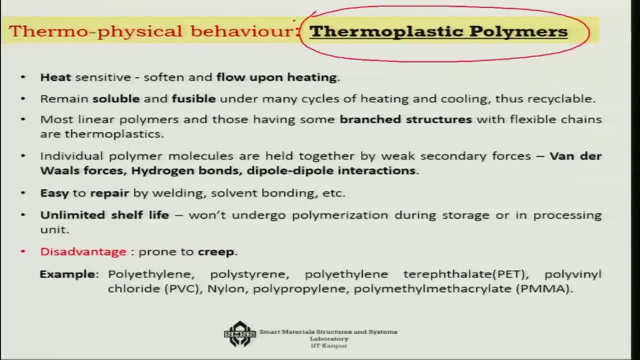 probability that it is a thermoplastic polymer. On the other hand, if it is- ah, you know- cross linked, or if it is networked, then it is more possible that it is a thermoset polymer. Now, thermoplastic polymers because of their nature, that they are, you know, linear, you know. 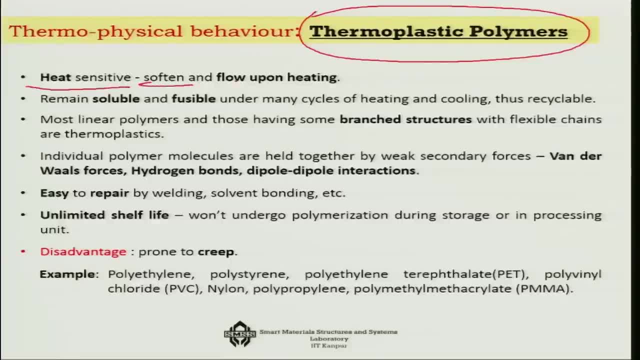 linear or, at most, branched. they are heat sensitive, they soften and they actually flow upon heating. It is very easily. one chain can smooth over the other, And I told you that they are soluble and fusible, and this under many cycles of heating and cooling. thus they are recyclable. 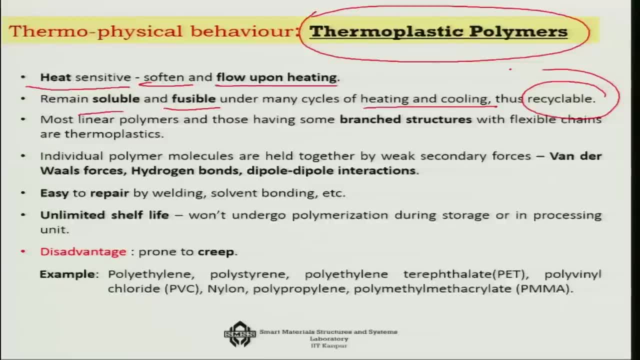 So thermoplastic polymers are greener in comparison to thermoset polymers, Most linear polymers and those having some branch structure. I told you already That these are actually thermoplastics. Now, individual polymer molecules can are held together, you know, by weak secondary forces. 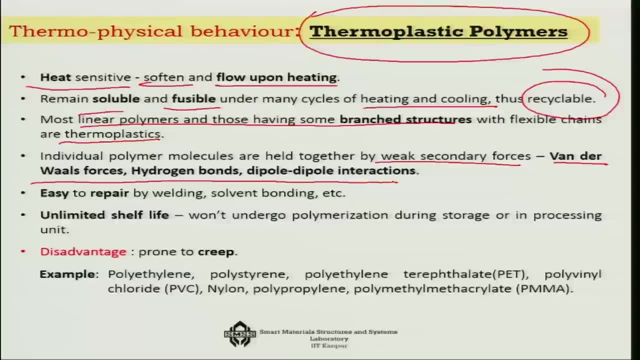 like van der Waals force, hydrogen bonds, dipole-dipole interactions. These are the general type of weak bonds between the two chains. So I have one chain and I have another one Between them. the force that actually works between them is either van der Waals force, 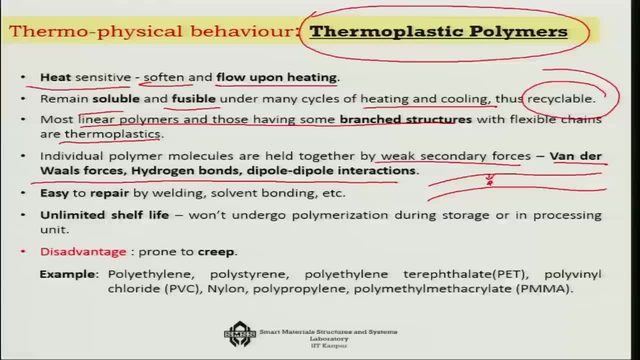 or hydrogen bond, Or dipole-dipole interaction, And these are all weak bonds. These are all weak bonds And that is why they are, you know, mechanically also they are weaker, particularly in the transverse direction, Easy to repair by welding, solvent bonding, etcetera, if there is a crack. because they 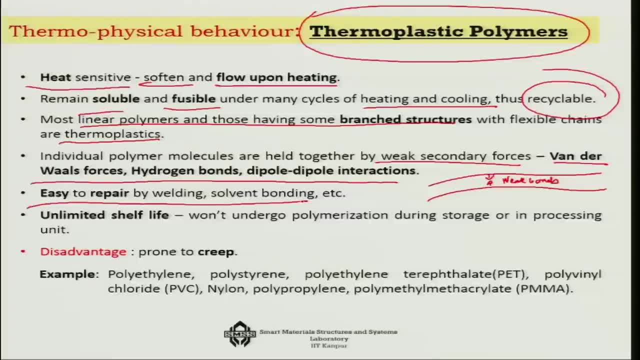 are formable, So you can actually apply a little bit of heat and then you can, you know, repair it. And also, very interestingly, They have unlimited shelf life. So you can actually apply a little bit of heat and then you can, you know, repair itAnd also, very interestingly, they have unlimited shelf life. 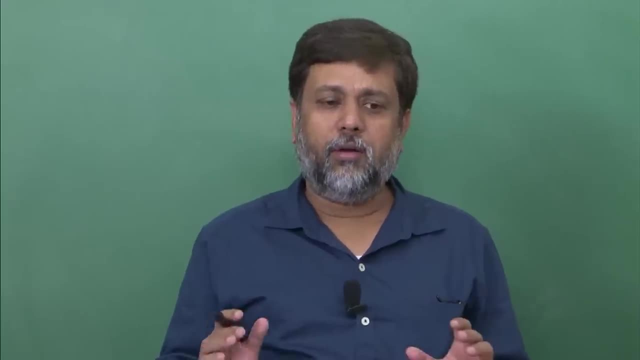 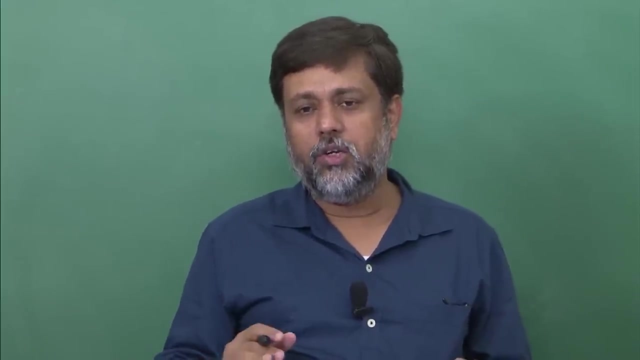 This is commercially important. Suppose: today I buy some monomer and then later on I think of polymerizing it. Now, for these monomers to polymerize and form a thermoplastic polymer is something in which you know at least it will not get set. It will not be completely useless if the polymerization suddenly starts, But you imagine that you have purchased that super glue from the market and you just forgot to switch to close it. What will happen? that there will be a polymerization reaction instantly as it comes out and get. 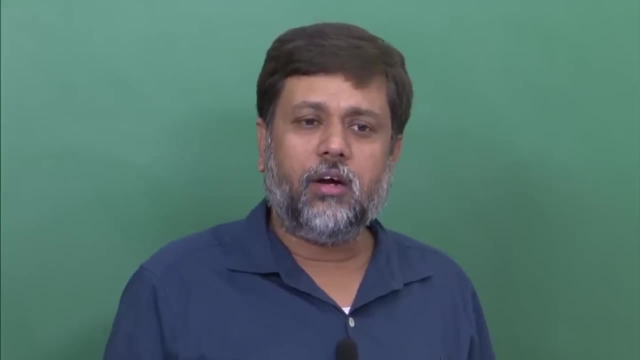 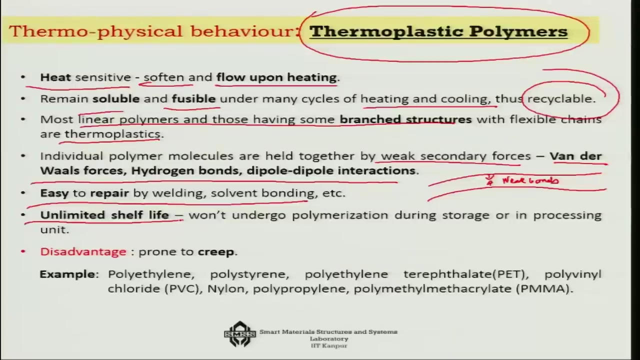 in contact of the air with oxygen, the reaction starts. So there will be, it will constantly, you know, get thermo formed, So it will become a thermoset And as a result that particular glue will be useless very soon. So then it has a very limited shelf life for the thermoset polymers, but thermoplastics do. 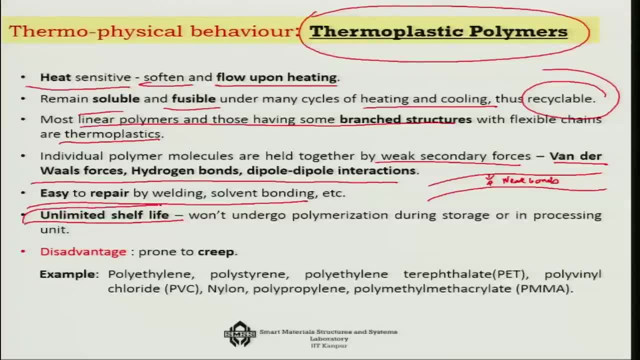 not suffer from this kind of problems. That is why you know it is almost like unlimited shelf life it is having. What is the disadvantage? It is prone to creep, Now that you can easily see that they, since the chains, can actually slip over each other. 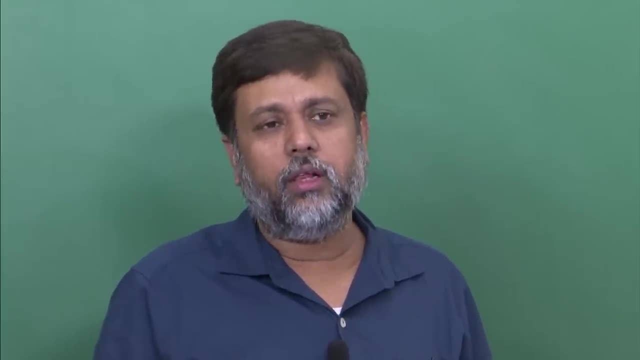 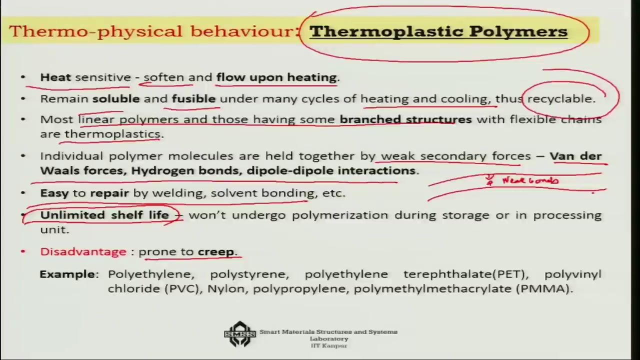 with a little bit of force, because the force that holds them together is a weak force, like van der Waals force or hydrogen bonding. Hence you know, it is a little bit of force, you can easily move one over the other. So the examples are like polyethylene, polystyrene. 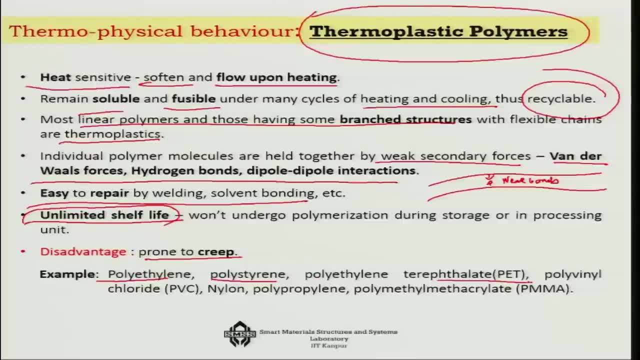 So you can easily move one over the other. So the examples are like polyethylene, polystyrene, polystyrene, PET that you see, you know many a times for using some of the bottles, etcetera, PVC's, nylon, polypropylene, PMMA, PMMA- one of the uses in your- you know- dentists, for example. 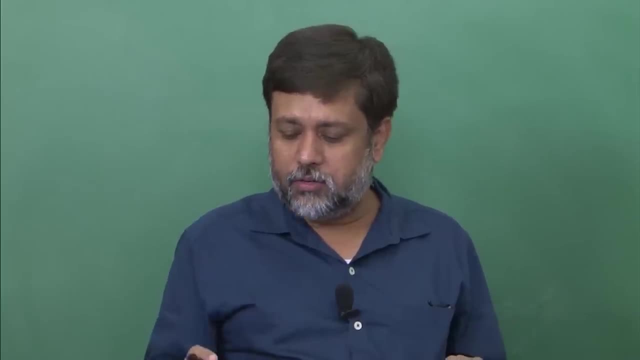 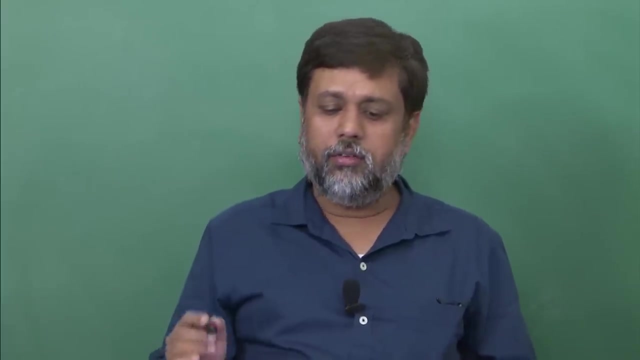 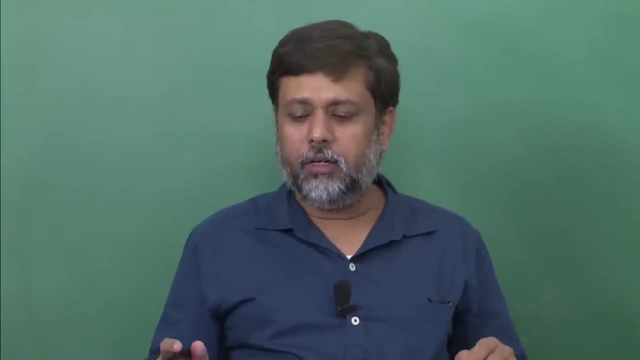 if you go, they actually make the teeth artificial teeth or such kind of using PMMAs. So you know it is also known as dentist's powder. So that is the thermoplastic polymers. Now let us look at the thermoset polymers. before we do that, what are the typical applications? 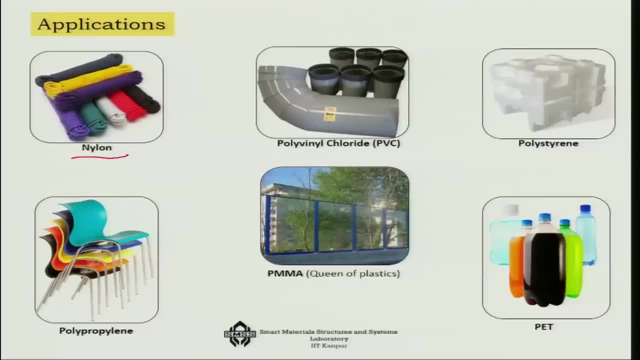 suppose, nylon. you know about the nylon wads and you also know that the nylon wads creep and the creeping happens because of the thermoplastic nature. then PVC's, polystyrene, which is used where there are more complex shapes, for example PMMA also, it is known, as you know, there is 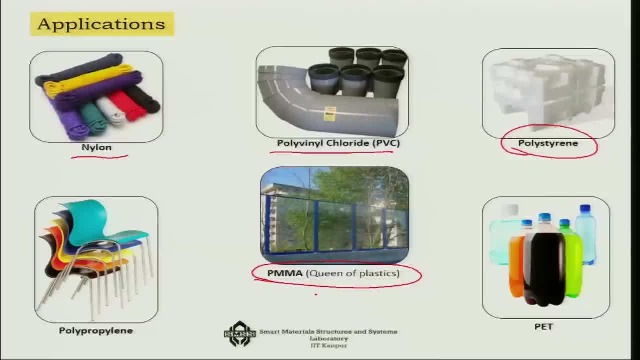 a common name of it. It is a call it. you know, Some people call it polystyrene, Some people call it acrylics actually. So you can, you know you will get it in the market as a artificial glasses, for example- they are transparent- then polypropylene, which is used in the chairs, for example, and then 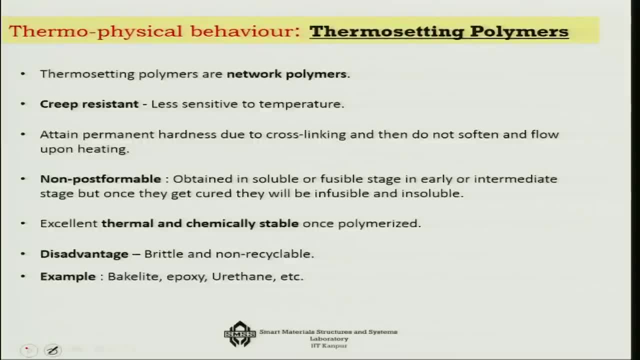 PET, which is used in the bottles. Now let us look at the thermosetting polymers. Thermosetting polymers are actually network polymers. they are creep resistant. they are less sensitive to temperature. The quite naturally, because, unlike the linear polymers, here you have cross bonding. that 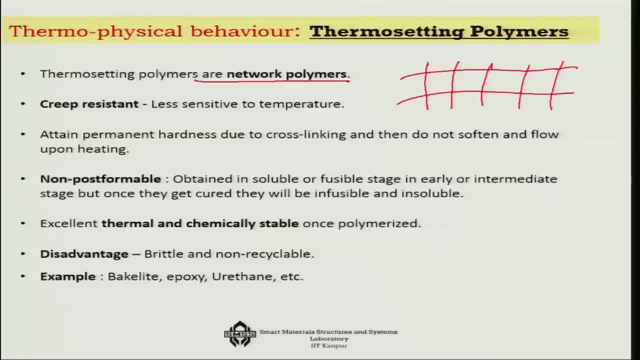 you have chemical bonding. That means the individual chairs are not very free to move with respect to each other. As a result, they are creep resistant. as a result, they are less sensitive to temperature and they attain permanent hardness due to cross linking. and once they attain that, once 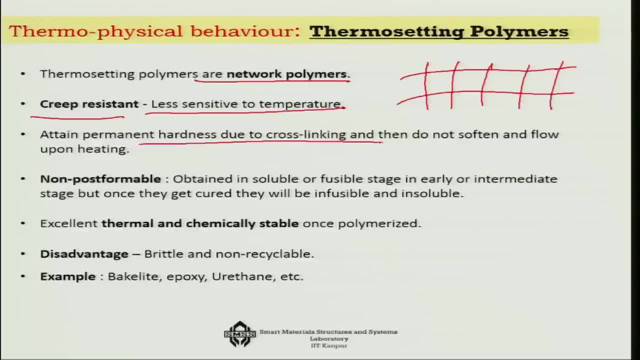 again, I want you to recall the super glue example. OK, Once it gets networked, then it do not soften and flow upon heating. that is the good part of it. but then that also means that it is non post formable. So that means obtained in soluble or fusible stage, in early or intermediate stage. but 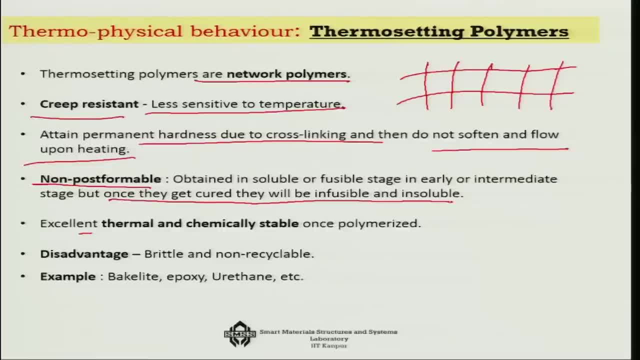 once they get cured they will be infusible and insoluble. So as a result, their shell life is actually very limited, and but the good part is that they have excellent thermal and chemical stability once it is polymerized. The mechanical disadvantageous part is that they are brittle. they are non-recyclable. 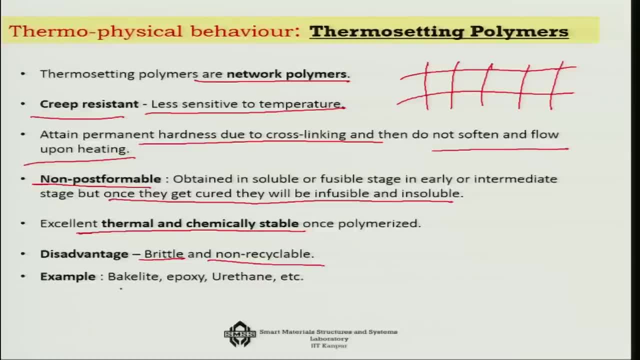 So that is the flip side of it, and the examples are like Bacallite, Epoxy's Urethane- Urethane is like the foams that you use in your sofa, for example, So that these are, you know, polyurethanes, PU. you call it PU foams. 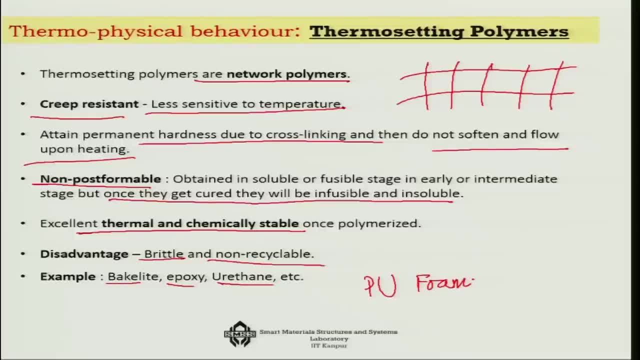 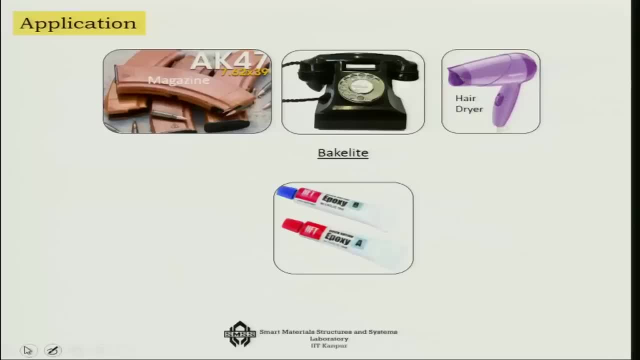 PU foam. These are very common name and that is used in your sofas, etcetera. So that is the thermosetting polymers. Now, in terms of applications, you can try to visualize. you know that it is used in the magazines, it is used in the Bacallite hair dryer. also, of course, the glues you know of. 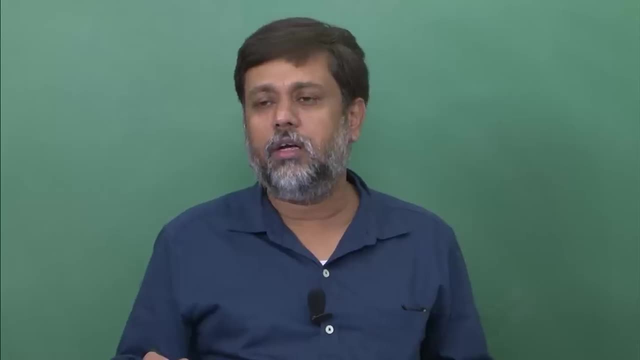 Epoxy A's, Epoxy B's. there are sometimes you will see in market that there are two kind of glues and you need to mix them together to actually initiate the polymerization reaction because they are so sensitive, the heat sensitiveness and the shelf life is so limited. 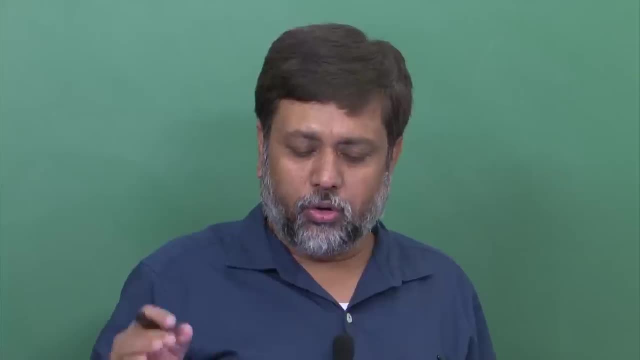 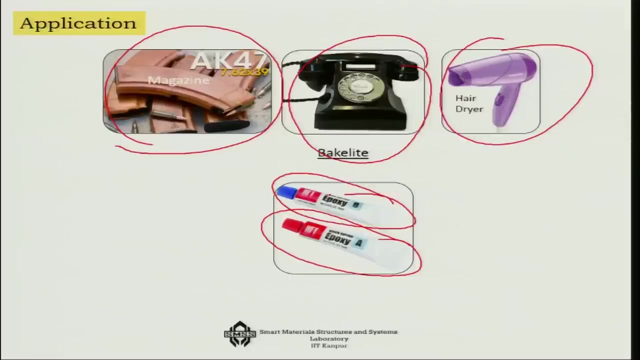 So its special care is taken that they do not automatically get you know networked like the super glues. So you will get them in two parts, like Epoxy A and Epoxy B. You mix them in a particular stoichiometric ratio, the polymerization starts. 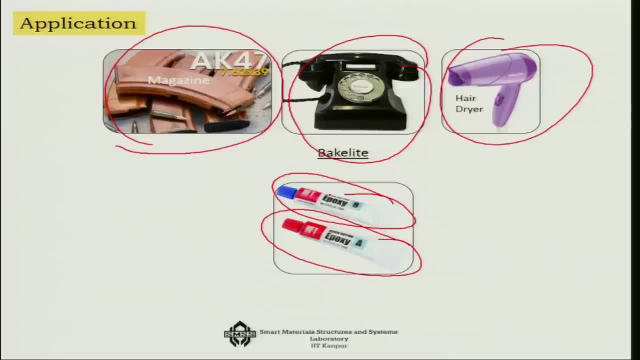 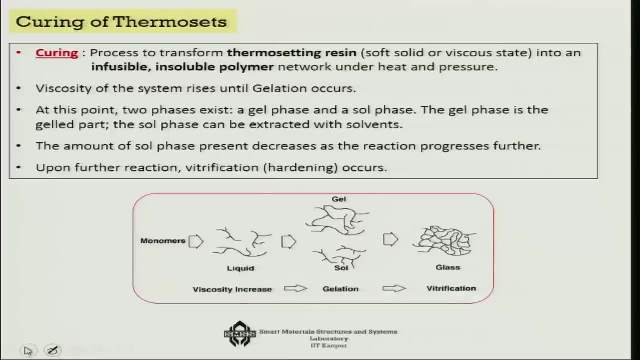 So you will get a good, hard thermoset polymer which is used in composites. Now, thermosets, that means it has to undergo a particular process called curing in order to get set. So the process to these you know from a monomer stage. first you are starting the process. 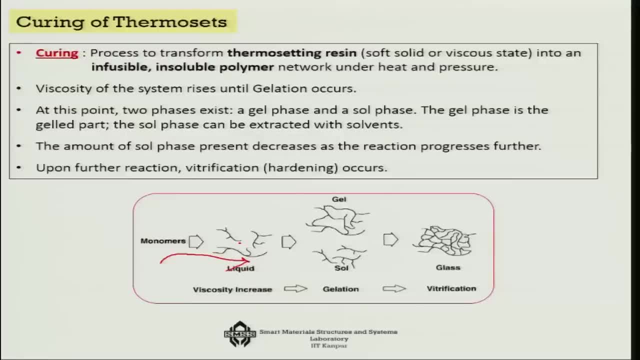 So in liquid stage itself the branching is occurring and then the gel is forming. So some are branched, Some are already chemically linked. So there is a sol and a gel phase and from there the amorphous glassy phase will start as you increase by the addition of heat and sometimes pressure. 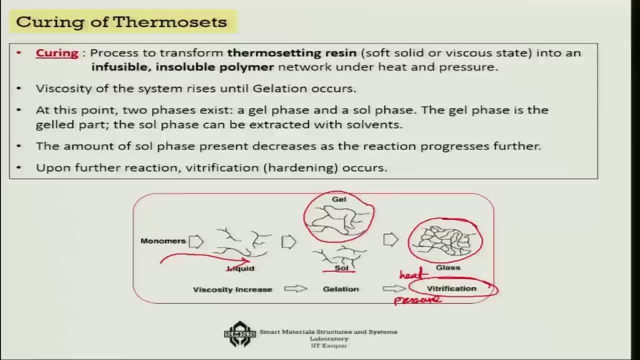 The gelation, the vitrification will start and you will get a fully cured thermoset. ok, So, over the time as this gelation is happening, The viscosity of the system will continuously increase and in between you will get that intermittent phase of gelation where you will get a gel phase and a sol phase, as I told. 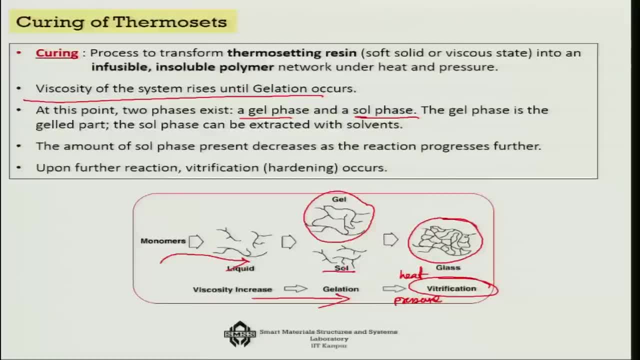 you and you know, with respect to time, the sol phase will gradually decrease and the gel phase will increase, So that basically you get all interlinked phases and then the hardening, or the vitrification, is going to occur in the system. The method in which we generally do it- I just want to mention it to you at this point- is: 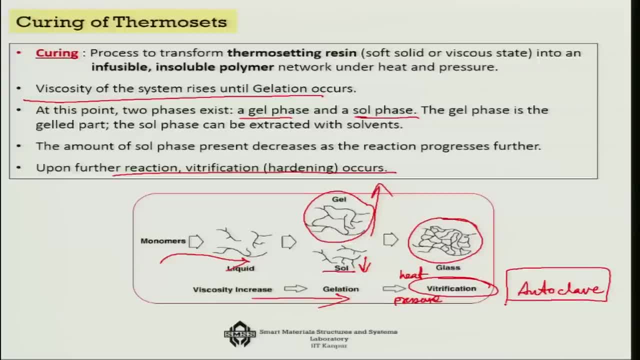 called an autoclave machine. ok, It is used, say, for example, when we make the aircraft wings. ok, So this is composite these days and in that composite, that matrix is nothing but a thermoset polymer. So that thermoset polymer is to be cured. 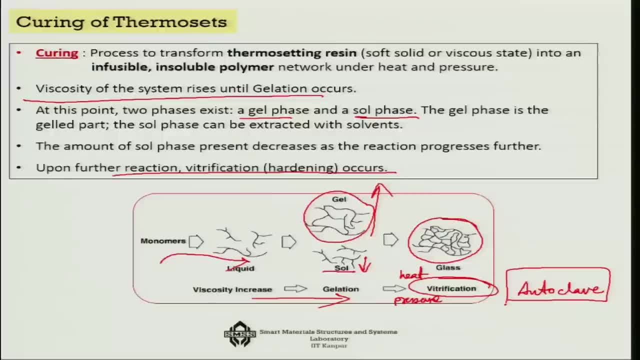 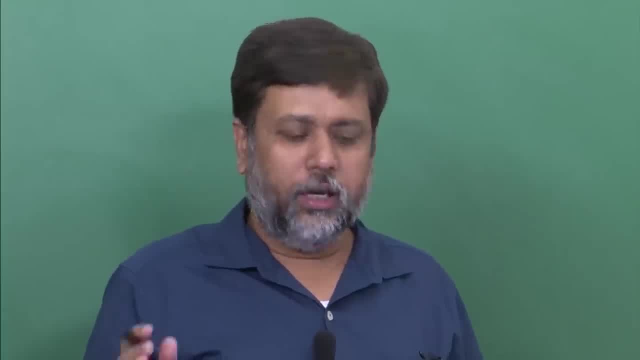 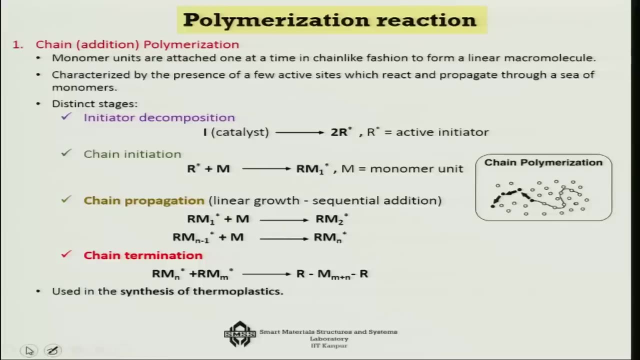 So what you do is that you actually make this whole thing out of a thermoset polymer and then put it under temperature and pressure So that it gets cured, the vitrification occur and you get that beautiful wing shape. Now what happens in this polymerization process? we have told many a times the polymerization 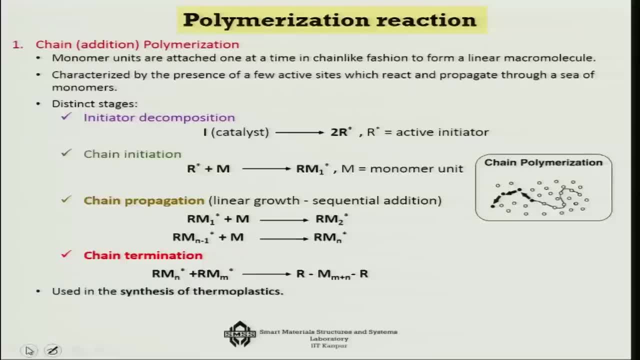 process from monomer to polymers. Now there are two types of polymerization process. one is called a chain or addition polymerization, So in this process the monomer units are attached to one at a time. There is a nearly 10st to 20 households in some 16ать. 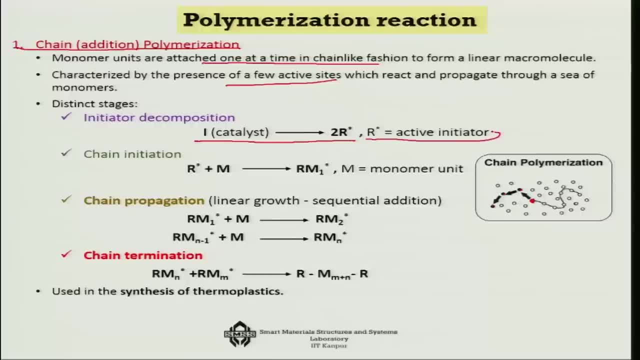 time in a chain like fashion To form a linear macromolecule. So there are only a few active sites in this case. compose, then the active initiator r star, will come this r star, the moment it is going to react with a monomer, you get the first active unit, that is the r m 1 star. then, as the chain, 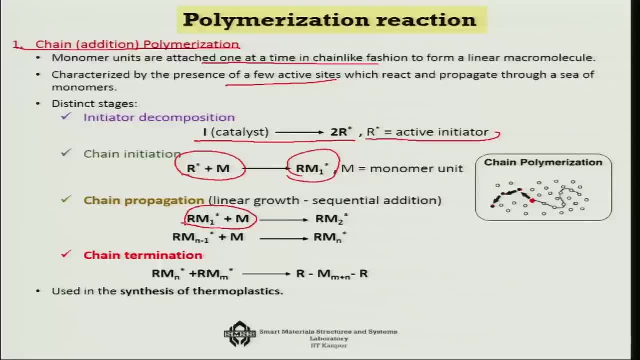 will propagate this r m 1 star with work with another monomer to get r m 2 star. then that process will continue, like one r m n minus 1 star will give you an r m n star. when that process will stop, when one of this r m n star is going to react with another of the r m 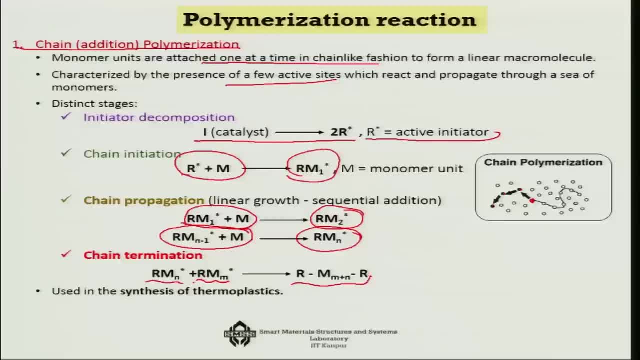 m star, then there will be a r? m? m plus n? r formation. So as both the sides are now of the polymer is having 2 rs, it will lose its cutting teeth. that means the chain polymerization will stop at that instant. So that is what is the addition of the chain polymerization. 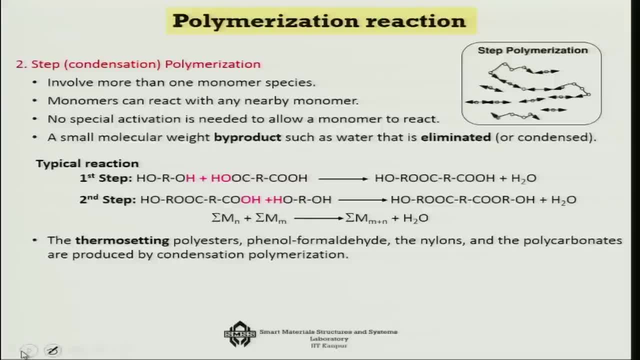 Much unlikely That. there is another type of polymerization where you do not have to really depend on one or two sides, but you can have simultaneous process of polymerization in many, many places. So you know like everywhere this is happening and this is like it can involve more than 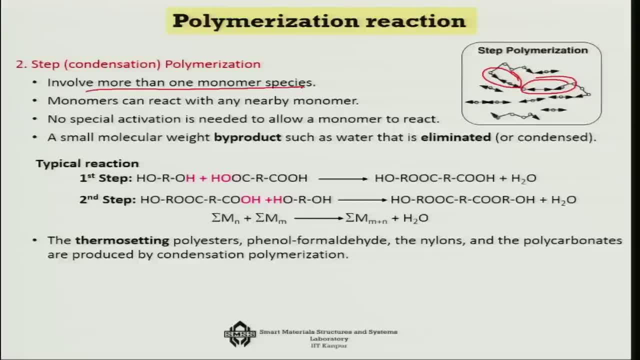 one monomer species and the monomers will react, you know, with any nearby monomer. they will not wait for, you know, some other active unit. So they will not wait for the active area to come and make them ready for the reaction. it would not happen. they will readily react. 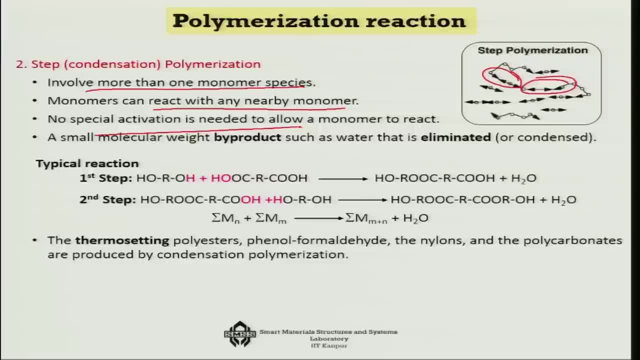 So no special activation is needed to allow a monomer to react and a small molecular weight by product, such as water, that will be eliminated. that is why sometimes this step polymerization is also called condensation polymerization. The typical reaction is like you have this OH element and then the. if this is a polymerization, 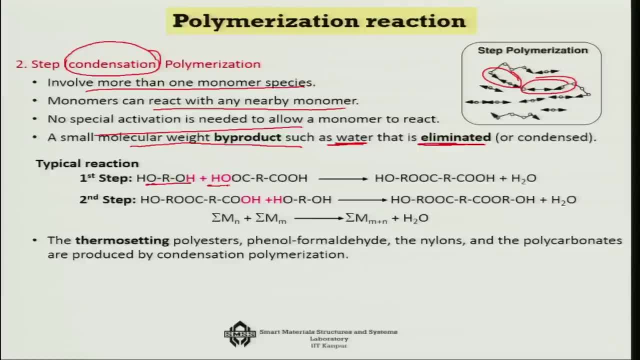 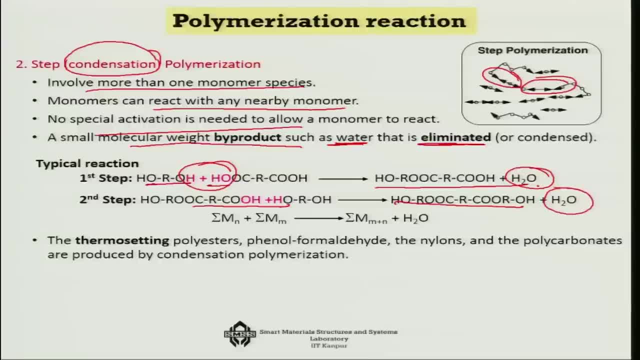 time you are getting some water or condensation out of the system. So that is, you know what is a step polymerization, And this you will find in polymers like phenol, formaldehyde, nylons, polycarbonates, polyglycines. 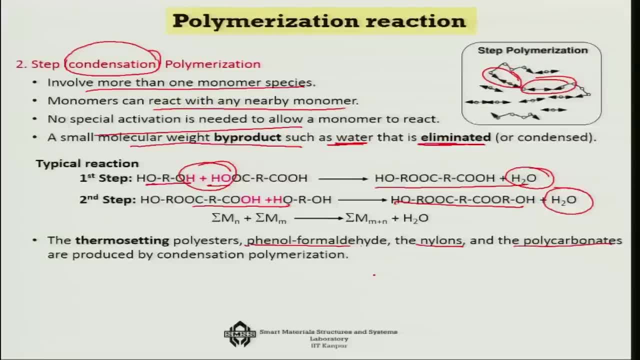 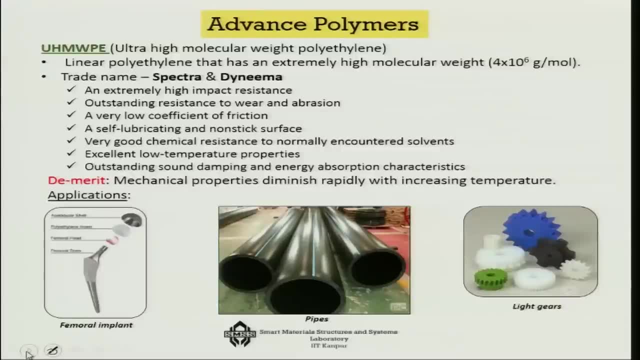 These are all produced by the condensation polymerization. Now we talk about some of the advanced polymers. One of them is ultra high molecular weight polyethylene like UHMWPE. This is becoming very important today because these are linear polyethylenes, but it has 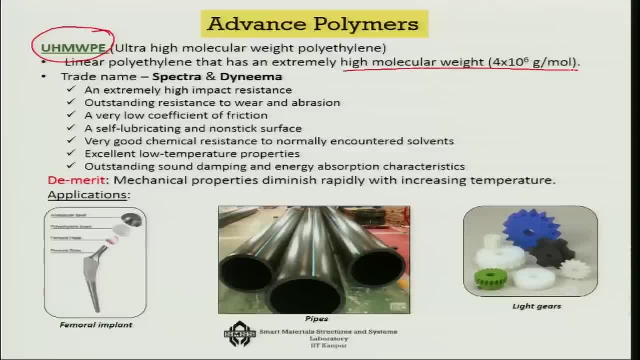 very high molecular weight. What is the significance of high molecular weight? That means you have, you know, the each monomer itself is so long that actually it gives you a high melting point, high mechanical, you know. it gives you a high modulus of elasticity, etcetera. 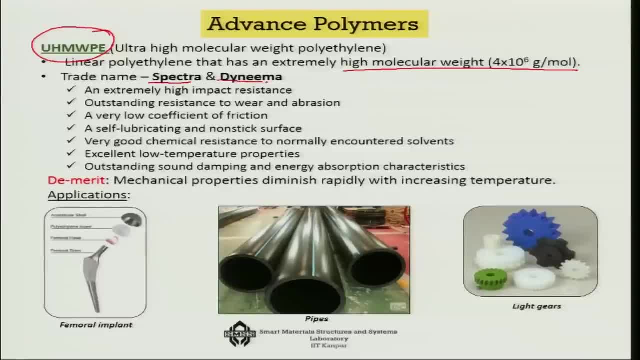 So there are two trade names of it. one is spectra, another is dyneema, and both of them have extremely high impact resistance, high resistance to wear and abrasion, very low coefficient. They are self lubricating and they have non-stick surface very good chemical resistance to. 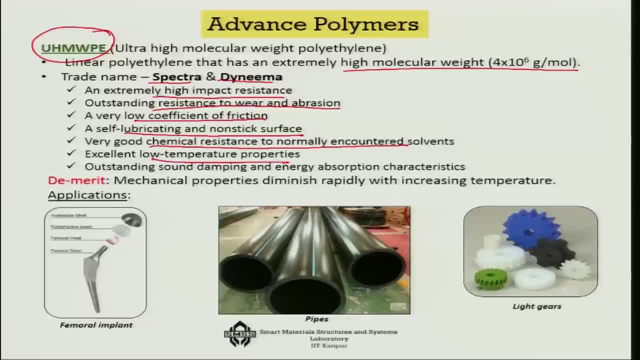 normally encountered solvents, excellent low temperature property and outstanding sound damping and energy absorption characteristics. Only thing is that their mechanical properties diminish rapidly with increasing temperature because they are, you know, the linear polymers, So they are susceptible to, as I told you, creep like problems. 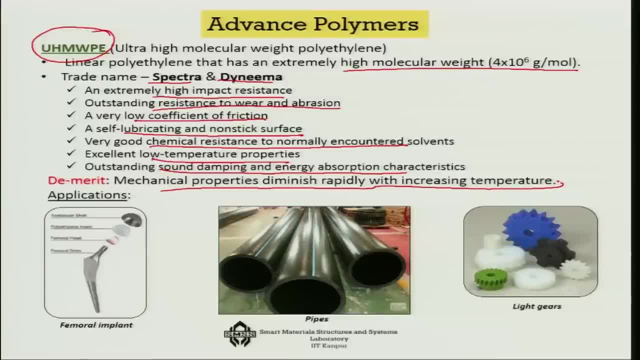 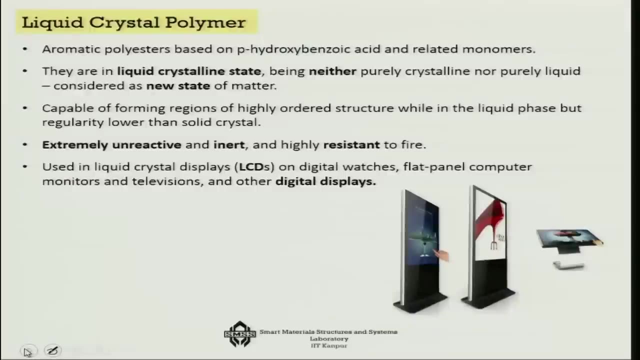 But at a. if a the temperature change is not very high, then they work. they have excellent properties. They are used in femoral implants, pipes, light gears in legos, etcetera. That is what one of the examples of a advanced polymers. 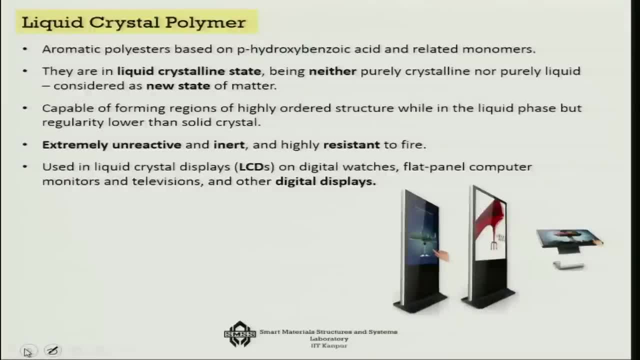 The another example of an advanced polymer is the liquid crystal polymers. So some of these aromatic polyesters based on, you know, PE, hydroxy benzoic acid and related polymers, they come into this category. Now why they are liquid crystal? you know we call it because in the liquid state generally. 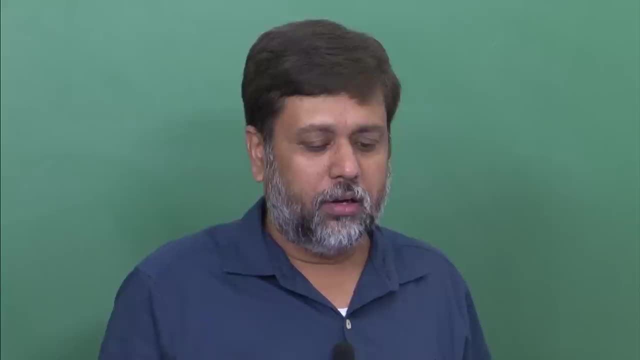 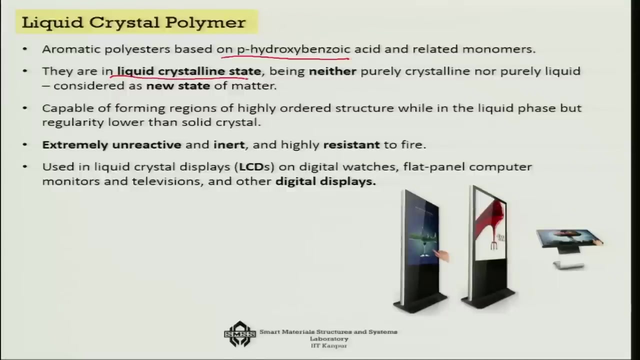 any. any material is supposed to be in a very amorphous state. But these materials, you know, in a liquid crystalline state you will get them. That means they will be neither purely crystalline nor purely liquid. So you can consider it to be a new state of matter. 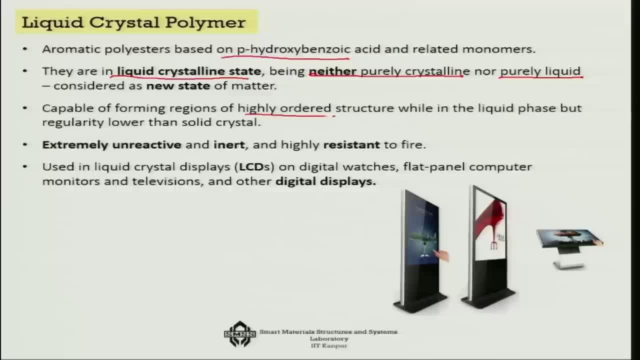 They are capable of forming regions of highly ordered structure, while in the liquid phase- But you know- regularity lower than the completely solid crystal. They are extremely unreactive and inert and highly resistant to fire. So something like your LCDs, the liquid crystal displays on digital watches, or flat panel. 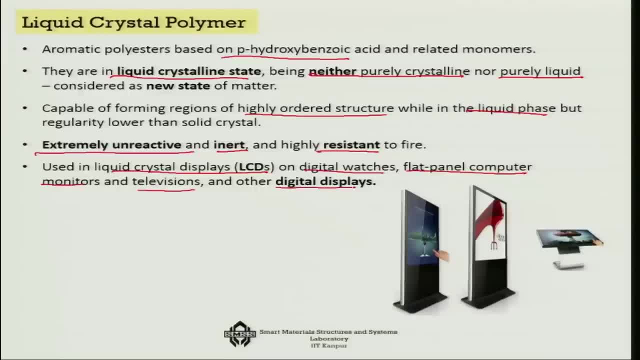 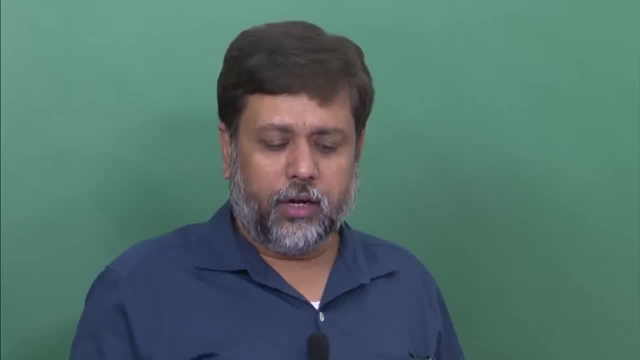 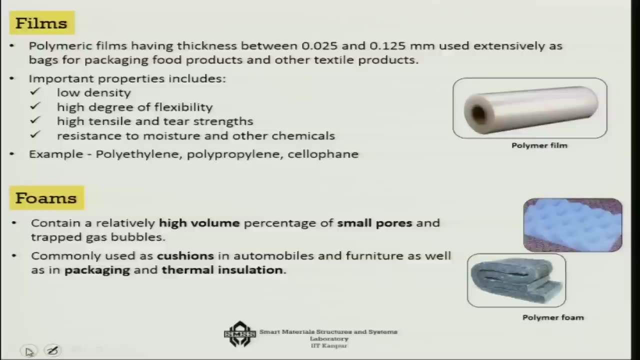 computer monitors, televisions and other digital displays. They are active. They are actually made of these liquid crystal polymers. Now let us try to categorize the polymers on the basis of the end use of applications. Let us see what are the end uses of a polymer. 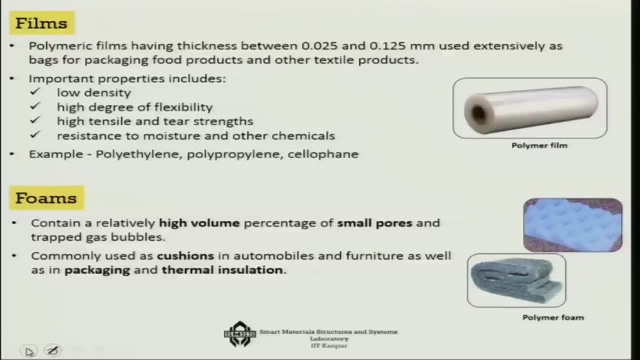 The first end use is in terms of the films. Polymeric films you will get in various sizes in the market from you know 25 micron. we also call it in terms of microns: 25 micron to 120 microns. 25 micron meter thin films that are used for packaging food products. 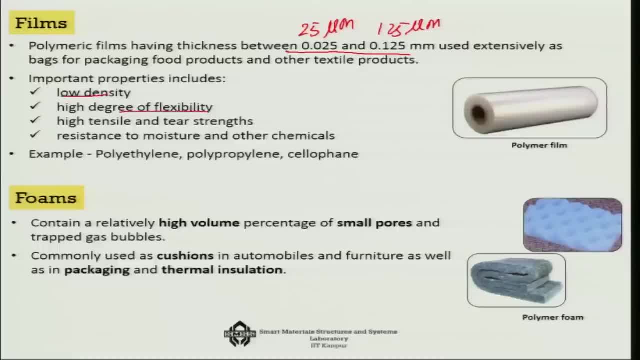 And their important properties. they are low density, high degree of flexibility, high tensile and tear strength, the resistance to moisture and other chemicals. That is why we generally wrap it up. So examples are polyethylene wrapper, polypropylene, cellophane, etcetera. 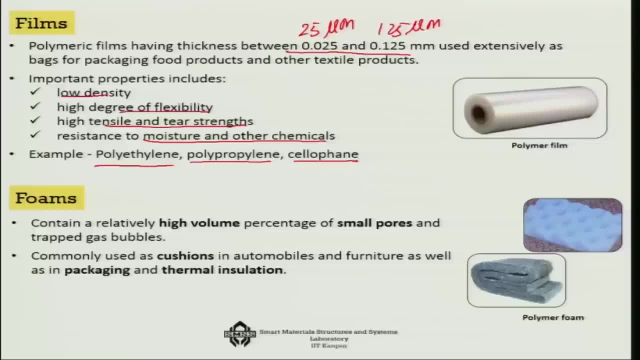 That is one group of polymers to where it is mostly used as films And other group. I told you about these. you know foams, right, the sofas, for example, which has the foams. So there you have the polyurethane foams. 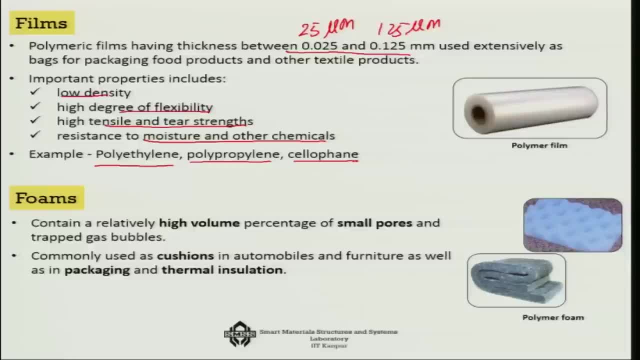 So foams are another very important categories of polymers. They contain relatively high volume percentage of small pores and trapped gas bubbles. They are commonly used as cushions in automobiles and furnitures, as well as in packaging in thermal insulations. you know, you get the polymeric foams. 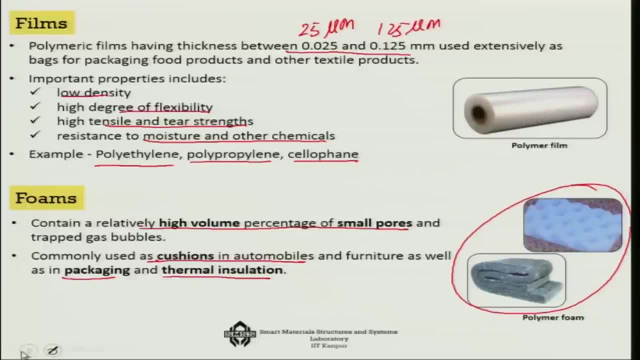 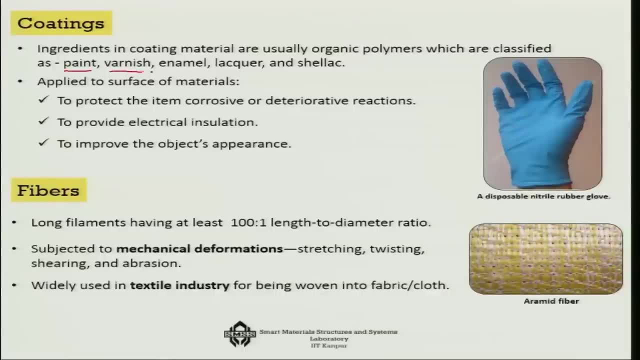 So that is another end use. so foams and foams. what else you will see? You will see polymers in coatings, for example in paints, varnish, enamel, lacquer and shellac. you will see them And they are used on to protect the surface and so that it protective from corrosion. 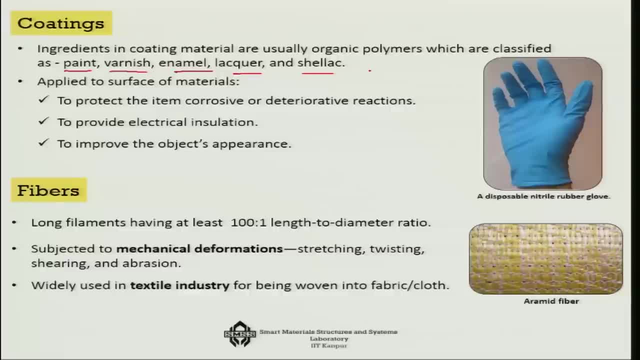 and for in electric insulations, to improve the appearance of an object, You apply the, you know, polymer colour, polymeric colours. so that is there for the coating, The very important use of polymers. suppose you consider a silk shawl, So it has silk fibre in it and the fibre is very, very important application of a polymer. 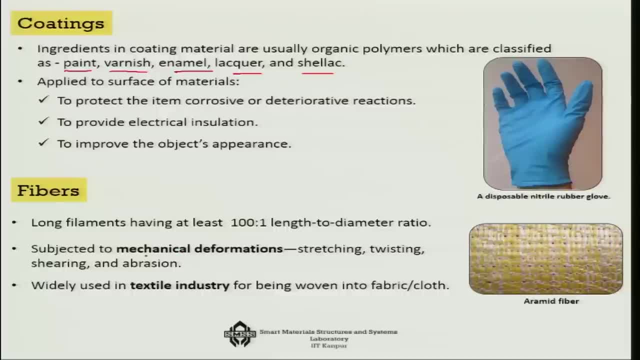 because it you know it has a very high degree of actually modulus of elasticity. it is an isotropic And you can use it for various applications, including making jet aircrafts right. So they are usually long filaments having at least 100 is to 1 length to diameter ratio. 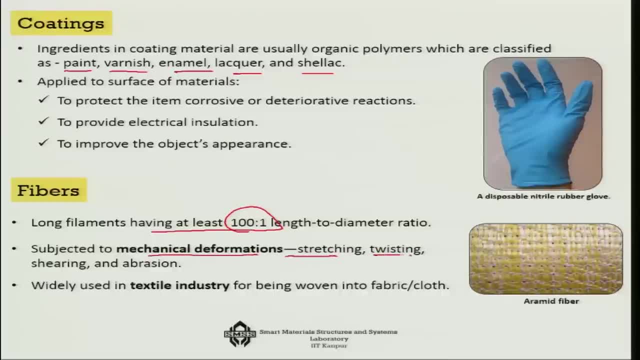 And you can subject it to mechanical deformations like stretching, twisting, shearing, abrasion. they are very good to absorb this. They are used in textile industry for fabric cloths, which can be either woven or it can be used to make composites. 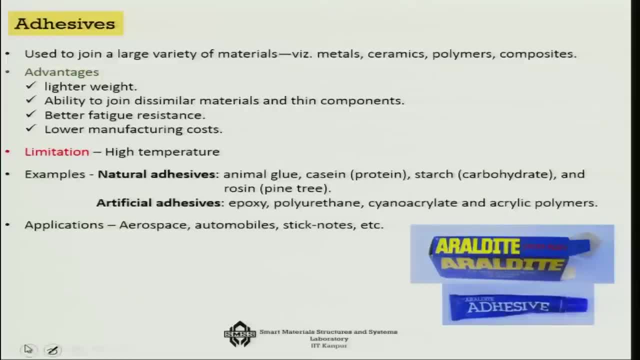 Thank you. Our next example of polymers is the adhesives. they are used to join a large variety of materials like metals, ceramics, polymers, composites, etcetera, And the advantage is that they are lighter in weight. they have the ability to join dissimilar. 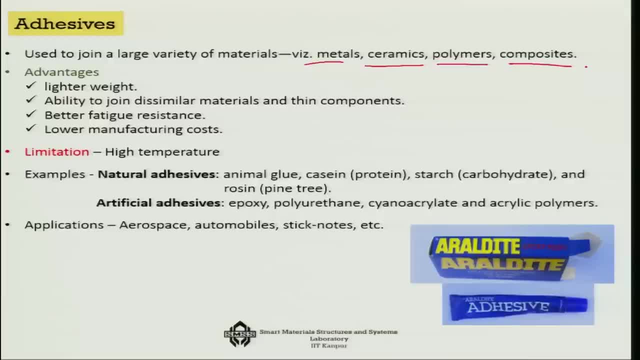 materials. they have better fatigue resistance and they have lower manufacturing costs, But the limitation is many a times in terms of high temperature or in terms of, you know, in terms of impact resistance. so these are some of the problems with a, you know, polymeric. 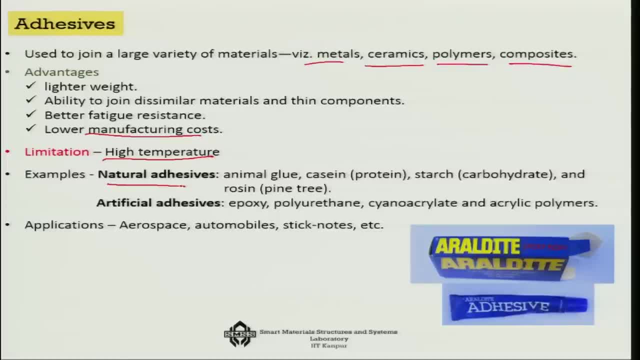 adhesives. There are natural adhesives like animal glues or caesines or protein starch and resins- ok, resin here- And artificial adhesives like epoxy, polyurethane, cyanoacrylate or acrylic polymers. they are 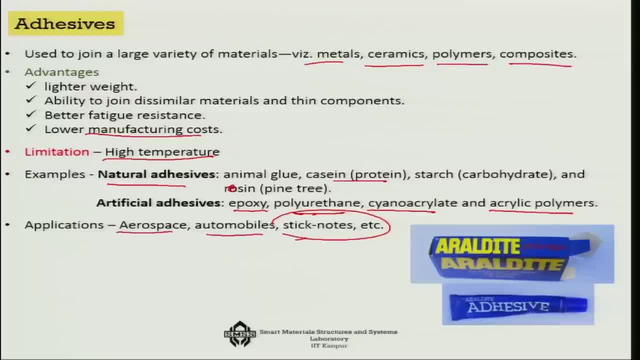 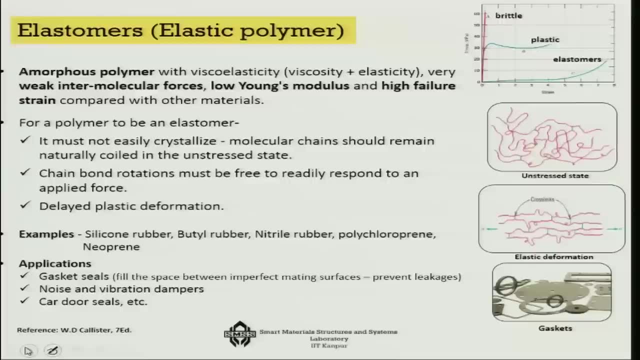 used in aerospace, automobiles and various types of stationary. Thank you, Thank you, Thank you is etcetera. So that is also become very popular use of polymers as adhesives. Then there is a good group of polymers which we call them to be elastomers. Now, what does? 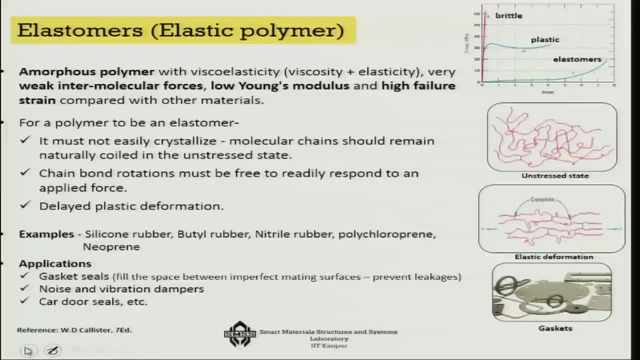 that mean? It means that they, if you look at this particular diagram, it will be very clear to you that any brittle material will show a high modulus of elasticity, but they will fail at a very low strain level. Now the plastics they will become, you know, non-elastic. 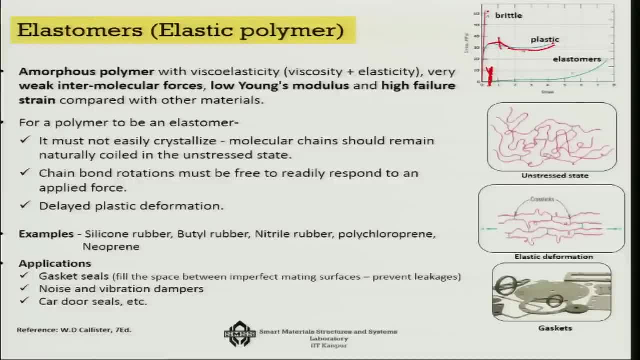 beyond a certain point, then the plastic strain will grow until it fails The elastomers. on the other hand, they actually remain elastic. that means if you actually unload it it will trace the same path, but they can take a very large deformation, So they remain elastic. 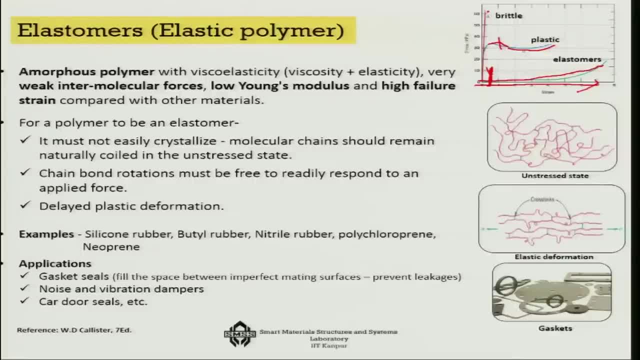 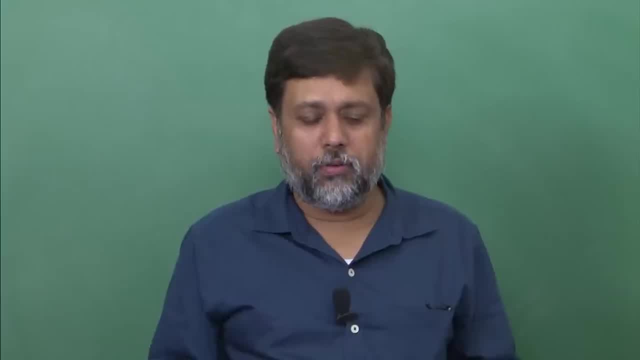 even beyond certain point. So they remain elastic, even beyond certain point. So they though in a non-linear manner, highly non-linear, but they can take up a very large, you know, strain. So naturally, whenever we talk of elastomers, what comes in our mind are the rubbers for 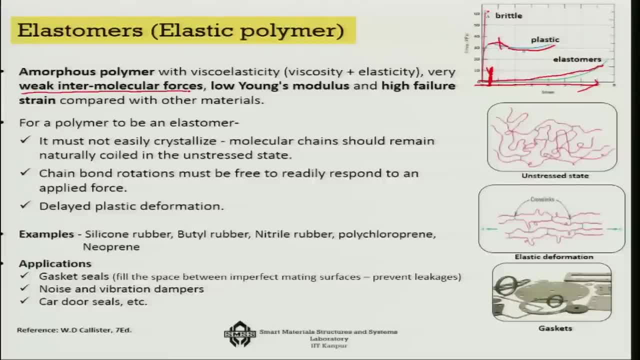 example. So they have very weak intermolecular forces, low Young's modulus and high failure strain. that high failure strain is very, very important for them. So for a polymer to be an elastomer it must not easily crystallize, because the molecular 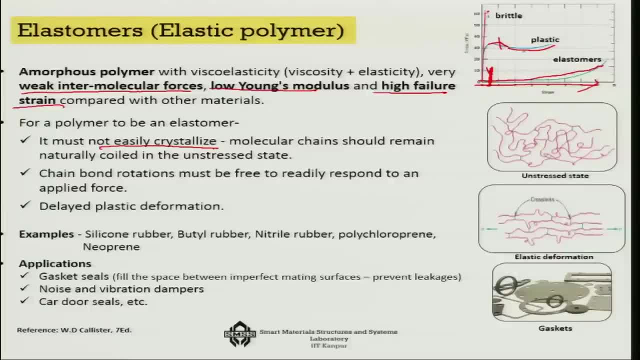 chain should remain naturally coiled in the unstressed state. The chain bond rotations must be free to readily respond to an applied force. delayed plastic deformation should be there. The examples are silicon rubber, butyl rubber, nitrile rubber, neoprene, etcetera. 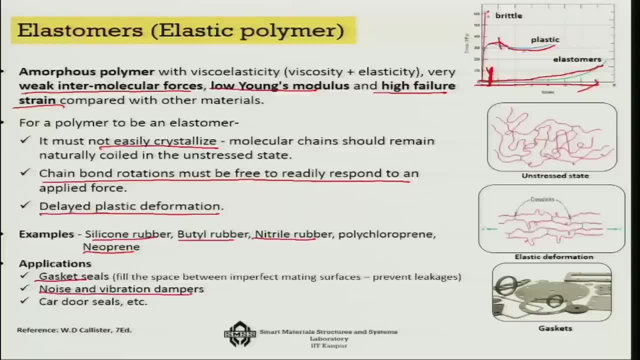 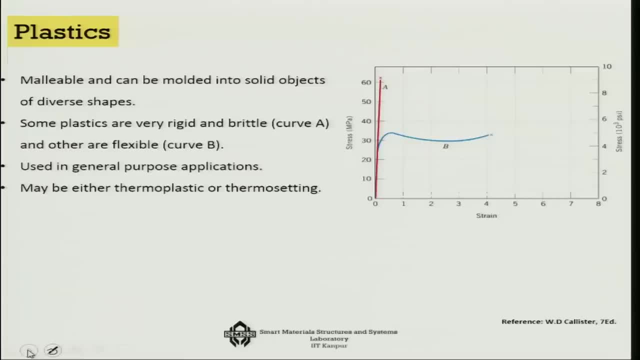 There are applications like gasket seals, noise and vibration, damper, car door seals, etcetera. So that is about the elastomers, The plastics. I already told you that this is like it is in between the elastomers and the brittle materials. 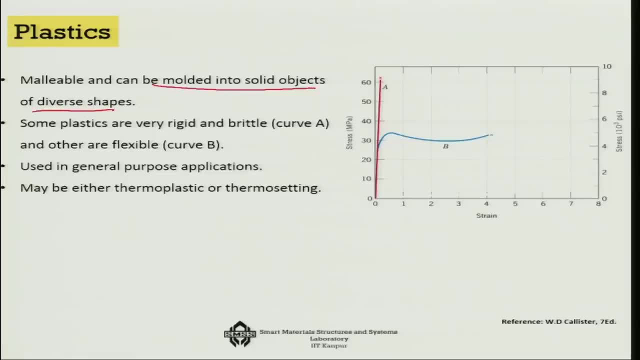 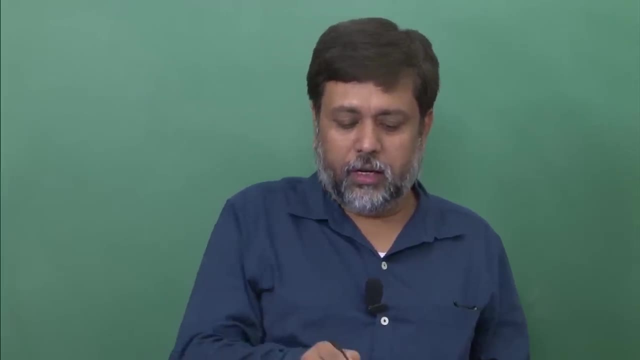 They are malleable, can be molded into solid objects of diverse shapes. Some plastics are very rigid and brittle and others are flexible. they are used for all general purpose applications, Like Some toys or very quick rapid prototypes. you want to make you use the plastics and they 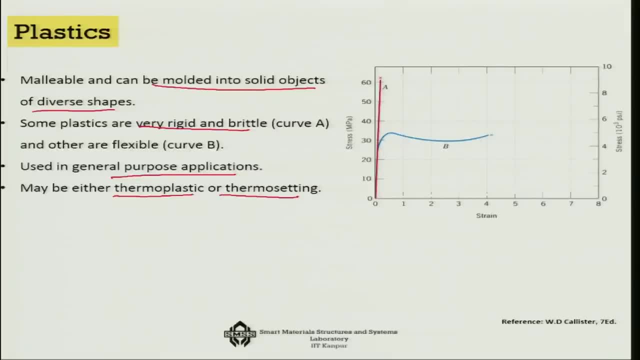 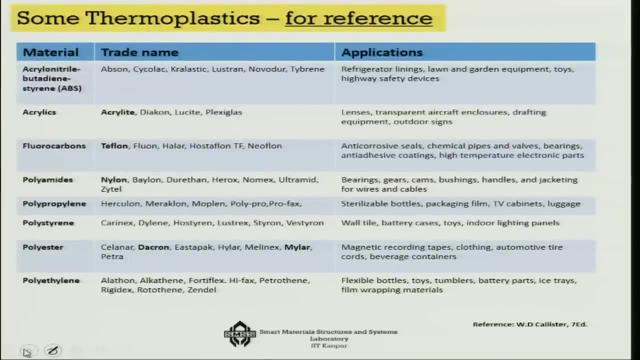 can be either thermoplastic or thermosetting. that is about the plastics. So let us try to keep some names of thermoplastics for reference, like ABS, which is used in all the what you call rapid prototyping purposes. So this is used mostly for rapid prototyping. rapid prototyping. 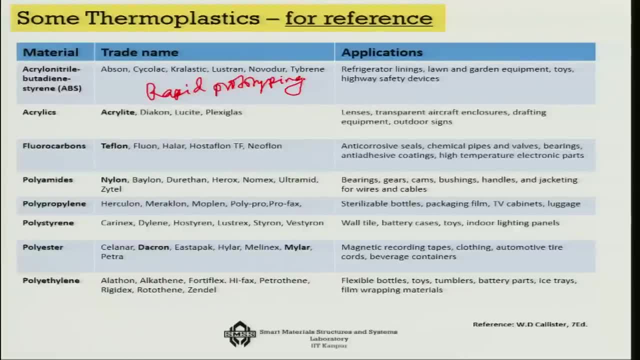 Then the acrylics I told you- the plexiglass is one of the examples- is used in lenses, transparent air packed enclosures, outdoor signs, etcetera. Fluorocarbons like teflon group, which is used in anti corrosive seals, chemical pipes and 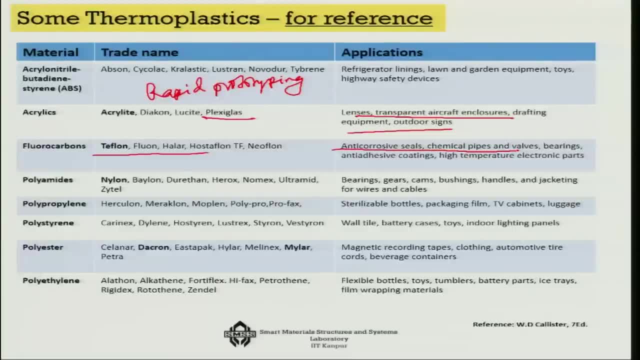 valves, because it is very much. you know, it is a high temperature resistant, anti corrosive material. Polyamide, like nylon group, used in bearings, gears, cams, brush handles, etcetera. polypropylene, which is used in sterilized bottles, packaging films, cabinets, you know, etcetera. polystyrene. 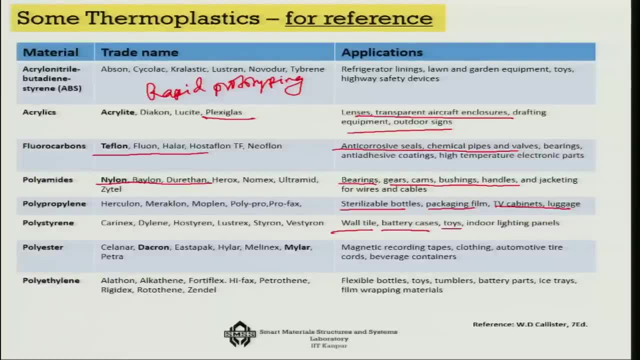 which is used in wall tiles, battery cases, toys, indoor lighting panels. They have a luster in them. Typical example is like Carinax, Dynex, etcetera, Polyester, Polyester, like this, you know, fibres, Dacrons, Mylar. they are used in recording tapes, clothing. 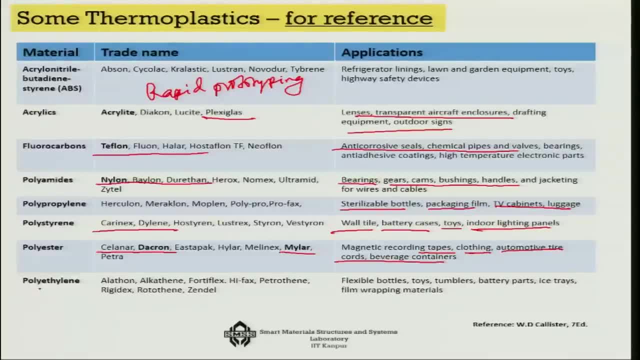 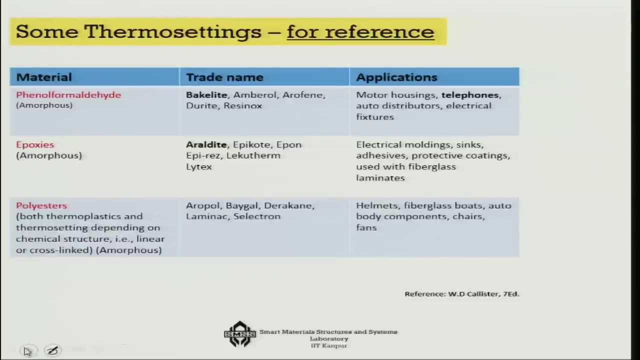 automotive tracords, beverage containers and polyethylene, which is, you know it very well, that is used in flexible bottles, toys, battery parts, tumblers, all sorts of very general purpose applications. Now there are the thermosettings, and there are three important thermosettings there. 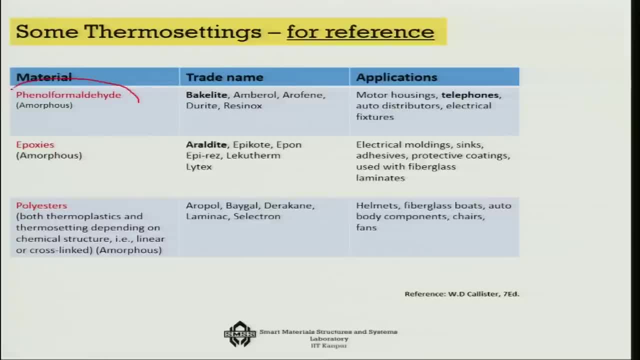 1. One is amorphous one, that is the phenol formaldehyde. the trade name is bakelite, it is used in, you know, telephones, motor housings, etcetera, Then the epoxies. it is also amorphous that the trade name, the popular trade name, is araldite.